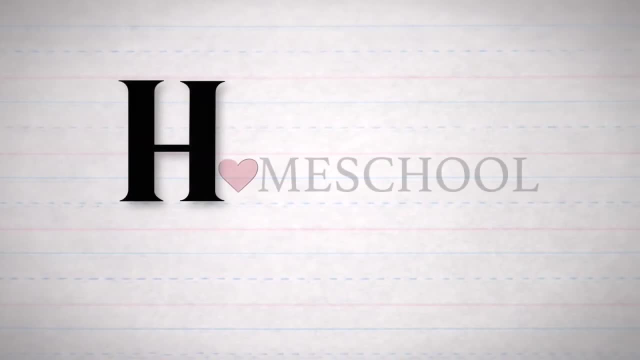 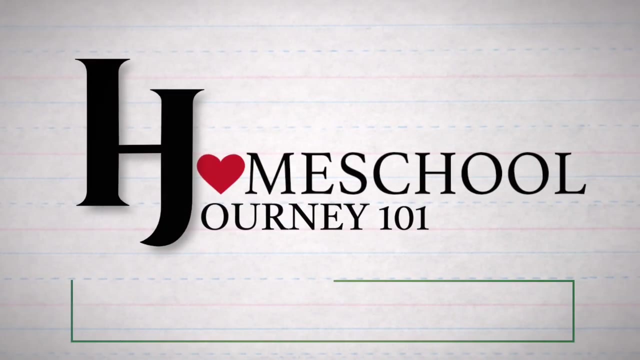 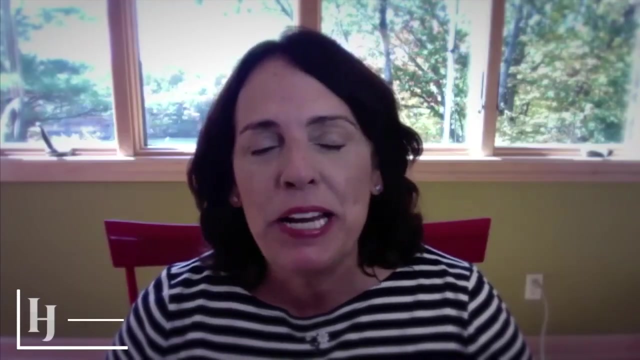 Hello, welcome back and thanks for watching. I'm Helen Hagen and my friend Rene Capuano will be joining us later. I was really inspired to make this video as a way to help parents with ideas to get their children away from screen time. 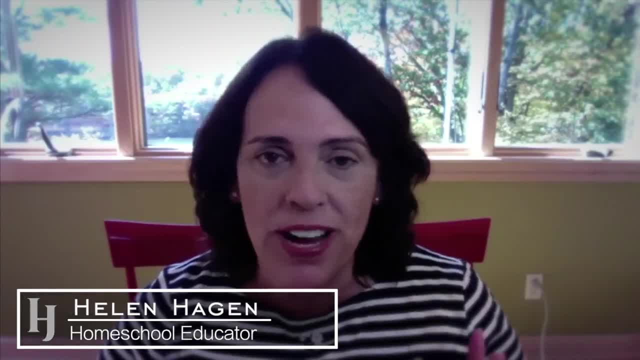 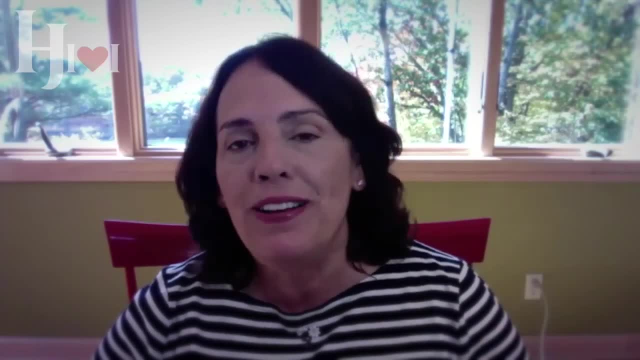 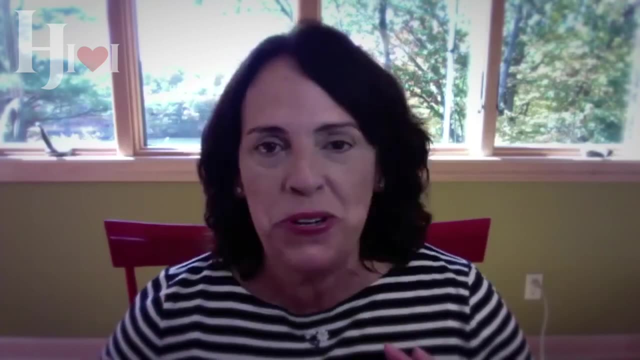 and to realize that even those young toddlers, even kids at one, can enjoy the great outdoors in big ways, in ways that will give them joy but will also build brain activities and build this love of nature, build this love of being outside and realizing the real world right, the real world outside of screens. 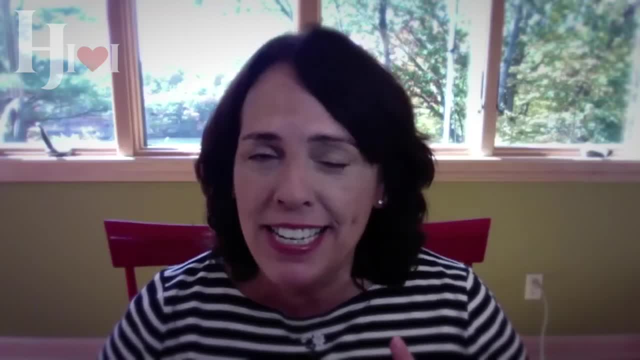 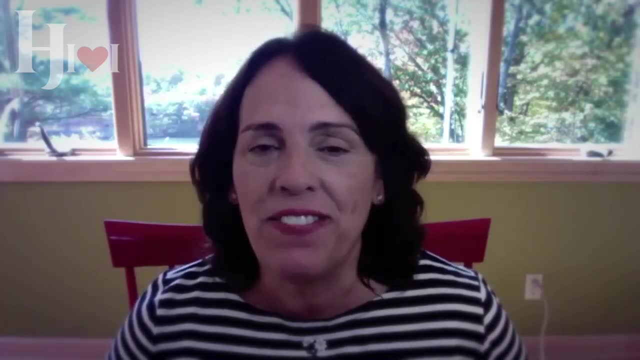 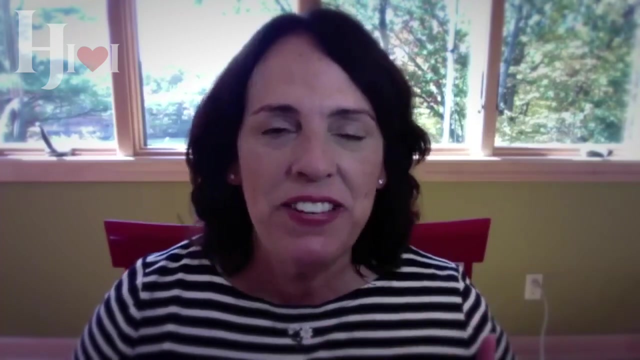 how rich that is and that builds different ideas, different contexts, different grasps of the processes that are going to be part of their life in a really different way than screen time. So I'm hoping that my years with my nine children, of all the different things that I have found to get kids to have that bond, not just with me- 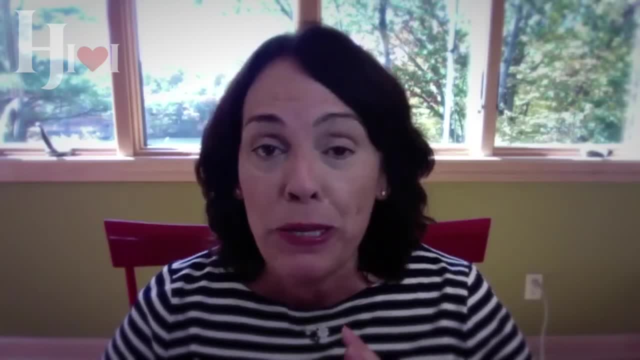 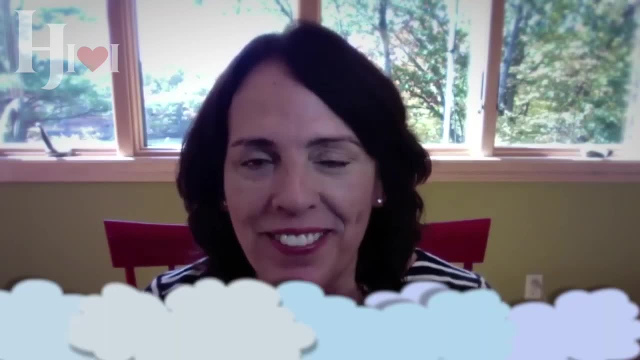 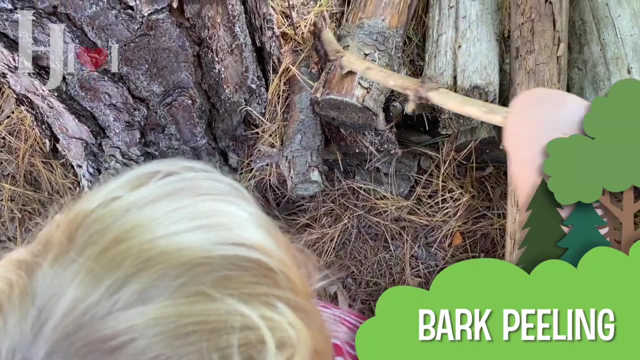 because I'm out there, too with them. So of course, it's really great at building family relationships too, but building their relationship with our gorgeous natural world around us. Okay, so let's get started with bark peeling. This is something that most of my children have loved to do, and the idea is: you have to find 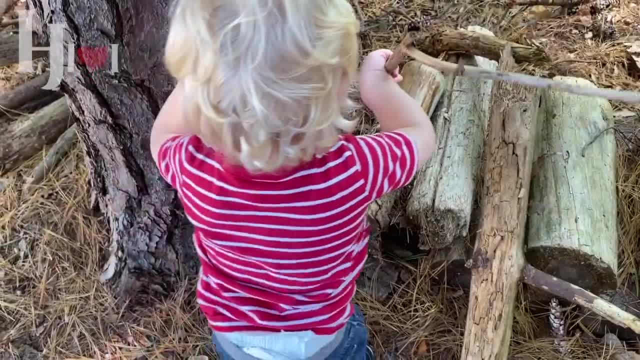 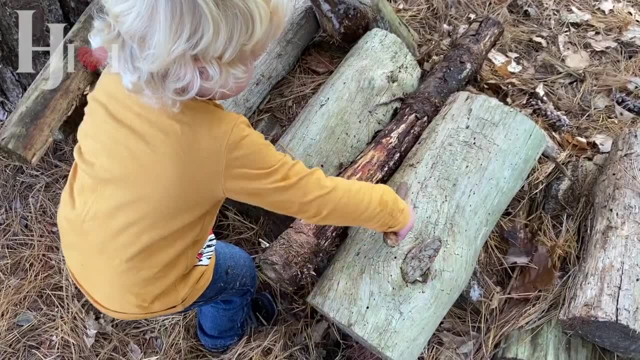 some logs that are already partly decomposed, partly weathered, and the child can use a stick- you can see here a small stick to just pry off of the, you know, a piece of bark, and it's so satisfying for them. 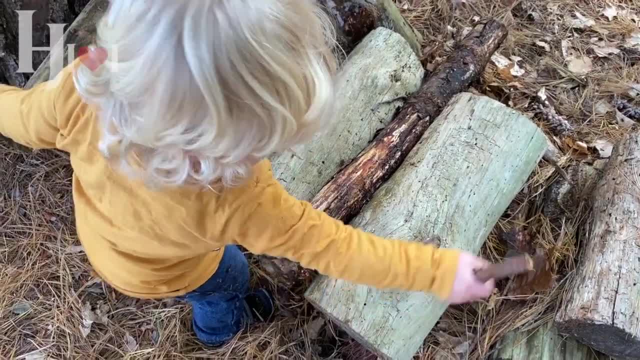 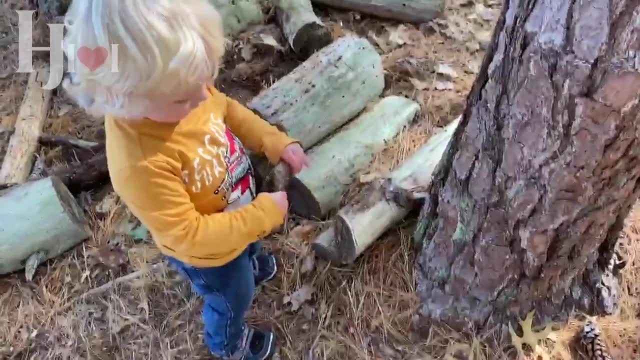 But also sometimes it's going to take a little longer. They can use larger sticks, they can use leverage. it's there's so many pieces here of learning how to pry things off lever actions and it's something about it is just kids just really love it. 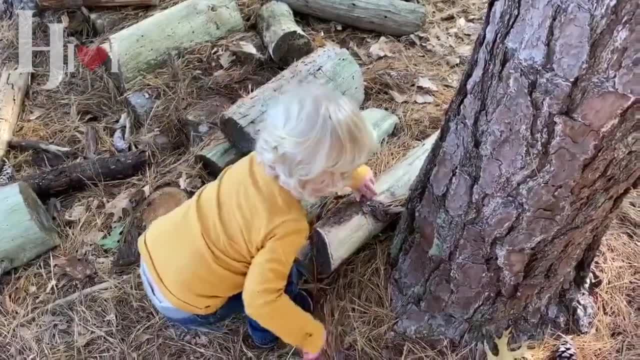 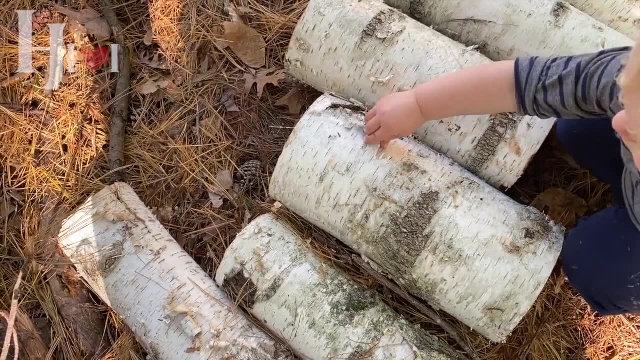 You can also use birch bark if you. you know, if you don't have access to Easy Nature, your birch bark is for sale. You know it's to look good on birch logs everywhere, And so the idea is just that they are taking the bark off. 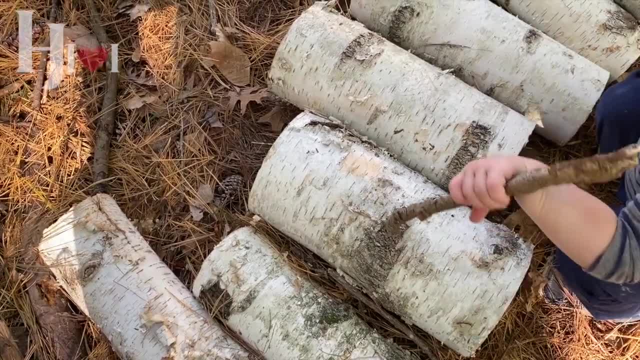 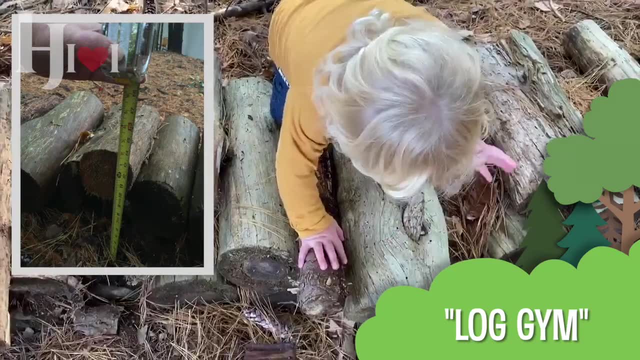 And so what that then builds into besides. yeah, that itself is very enjoyable, but is what I'm going to call a log gym, And so I use these with all of my kids, and it's important to notice that this is very short right. 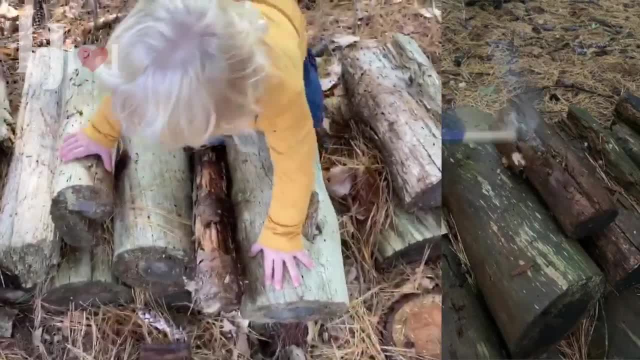 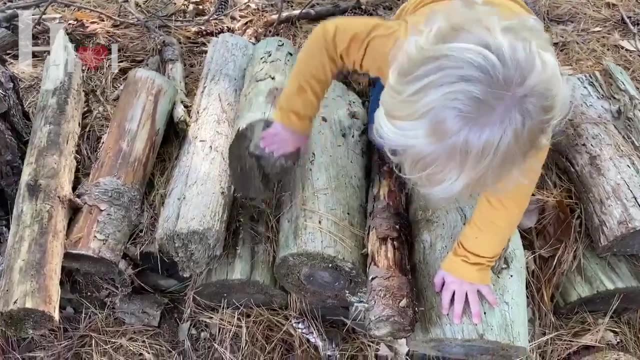 And if you use logs that are already, you know, partly weathered, partly decomposed, you can see here with my little hammer experiment, they really give. So they're much safer for the child, because even if the child hits their head, it hurts a lot. 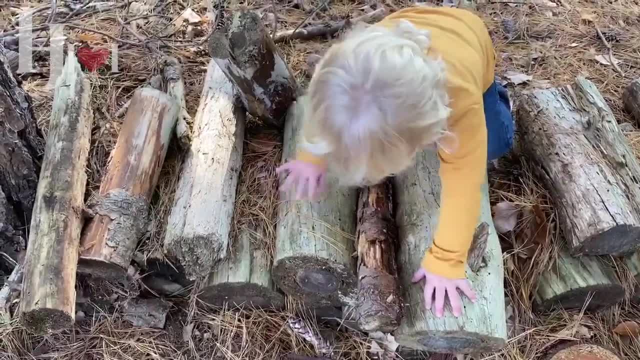 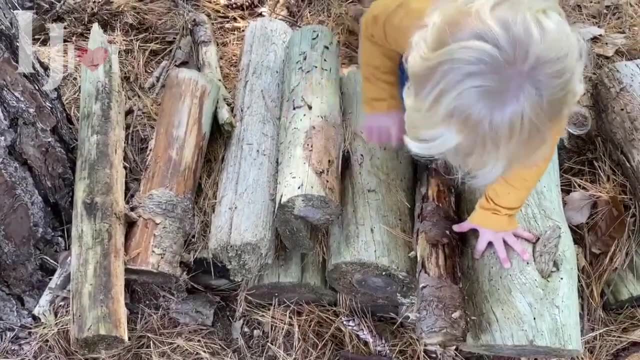 It's a lot less than a log that's just recently, you know, been cut. Okay, this is a lot more give in it, but also it's a lot easier to not get scratched up. But, yeah, wearing some heavy jeans and some closed-tipped shoes. 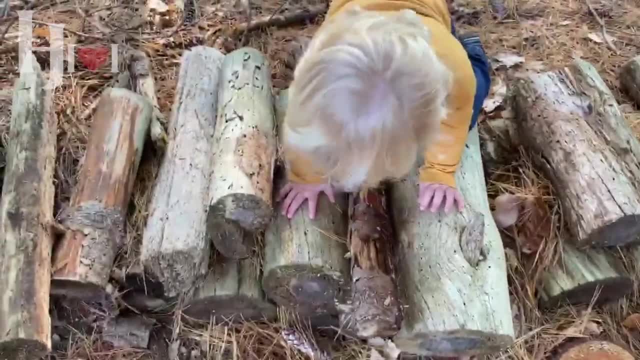 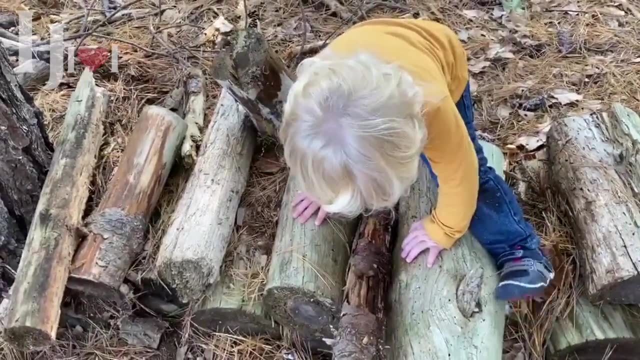 you can see that he is just having the time of his life, right, And I don't know if you can hear his many giggles here in the background, but this is something kids just love to do and it can be constantly changed. 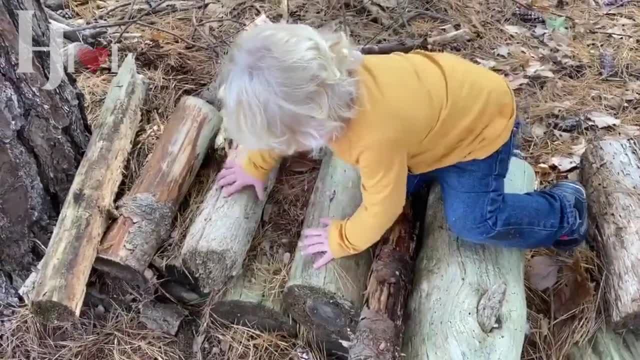 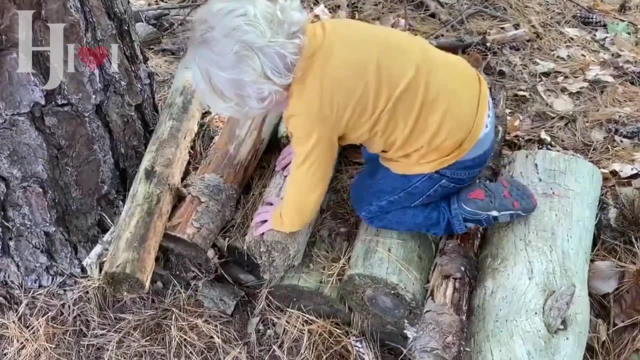 because you can move the log. Sometimes the logs move a little bit themselves. You see my hand in here several times because I do feel like with a young toddler I am right there behind him to keep him, you know, as stable as possible. 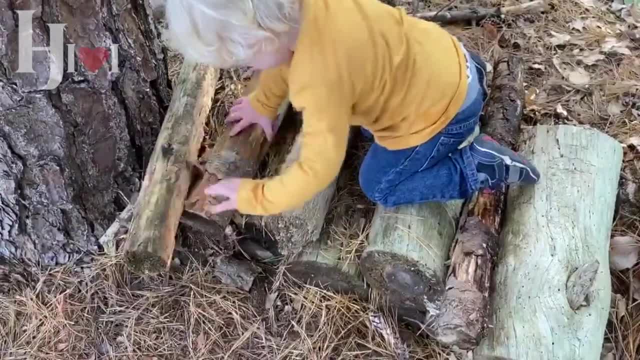 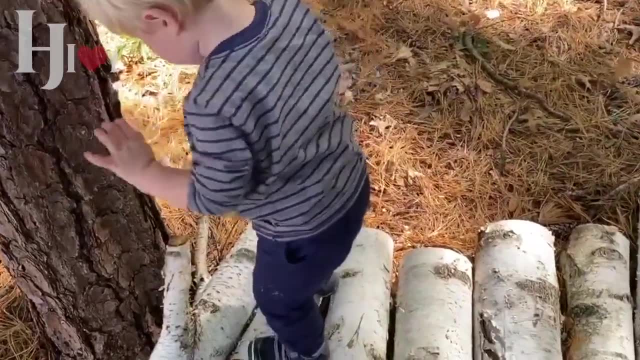 But he's also learning himself, like what works, what doesn't work, How can I climb up, How can I climb over? It's so fun for toddlers, It's just so fun. They love it. It's also great for coordination and it's great for thinking right. 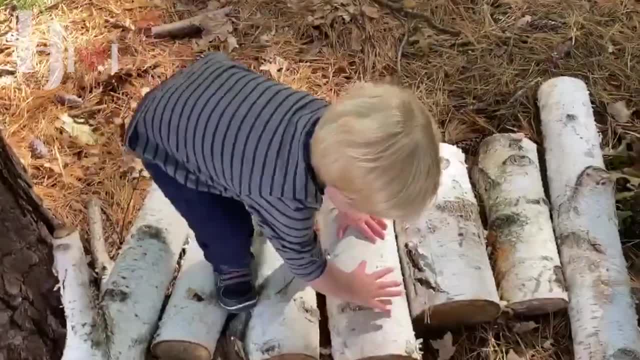 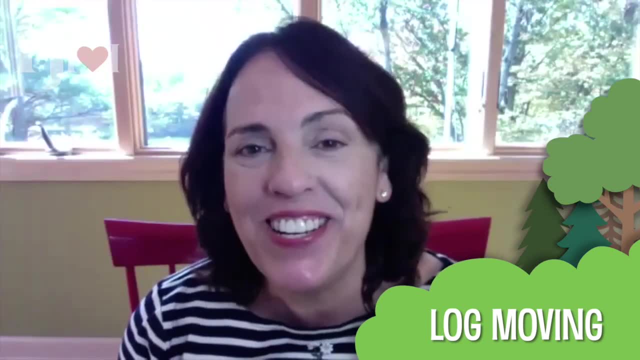 Like: how do I get from here to there? How does this work together? What do I have to do to move here? All right, I'm going to call the next piece log moving, And this is all the ways that your child can move these big logs. 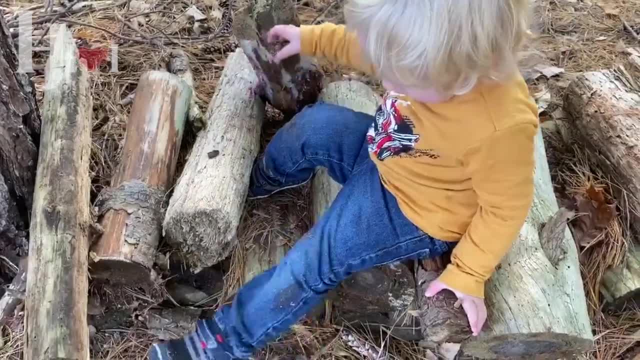 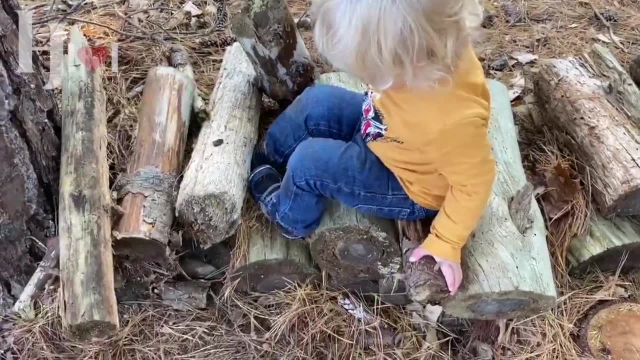 It's a real confidence builder. It's very interesting to them that they can take their whole log gym apart. So you can see that between these two trees he can take all the logs apart. He can put it back together and make his own interesting log gym if he wants to. 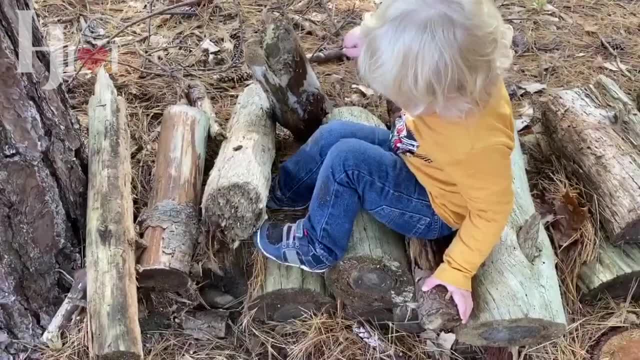 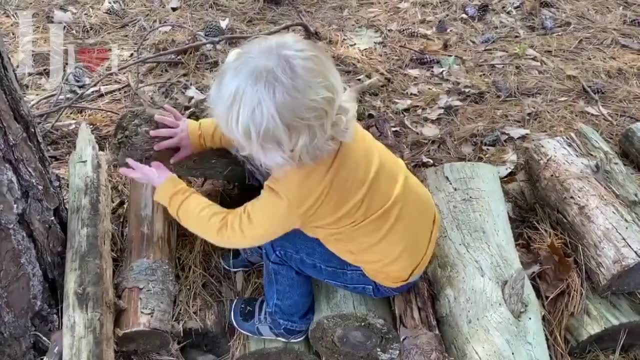 But also he can kick them over, He can move them over. You can see, here He can put his, He can put his feet under the actual logs, using it sort of as a lever. Lots of thinking in this whole experience of moving these things around. 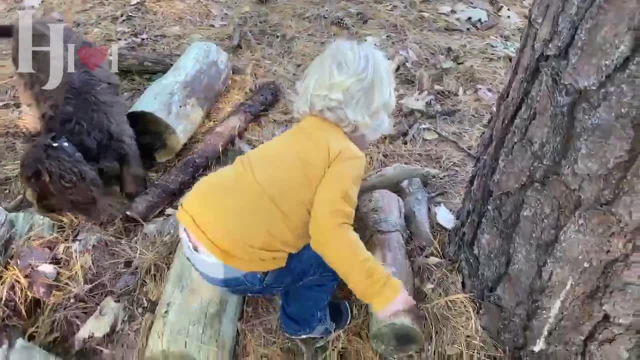 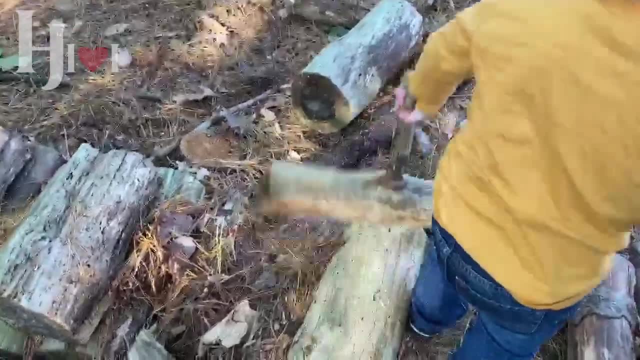 But it's also very joyful for him- You can hear him giggling- because these are big things that he can move around himself. Again, because these are these weathered logs that are much lighter than you know freshly cut lumber. All right, so the next one is: hit a tree with a stick. 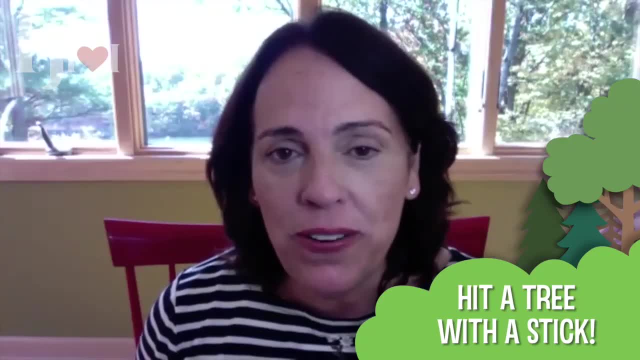 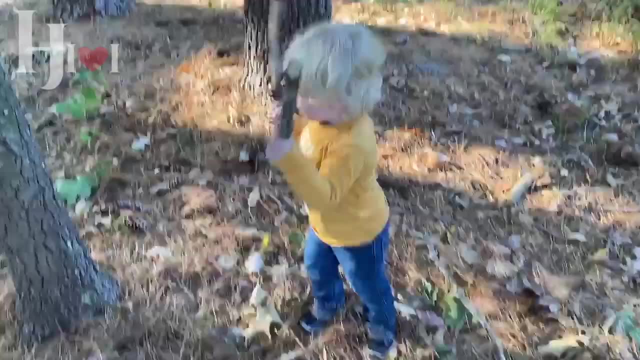 Now I know that this seems very surprising, But if you show a child this, there's something that's just so satisfying for a toddler and so intriguing that they can make that sound right And you can see he's just going up. 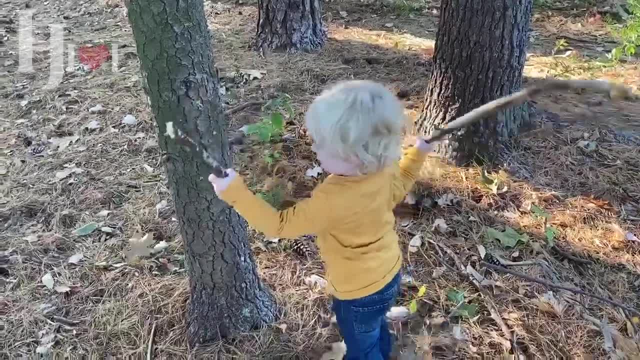 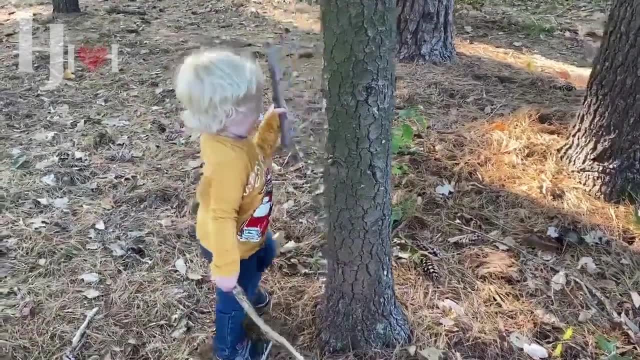 He's trying with two sticks. You just want to make sure they don't get going hitting it too hard, where they let go of the stick and they can hurt themselves. But this is something that kids love to do at this age. They just love it. 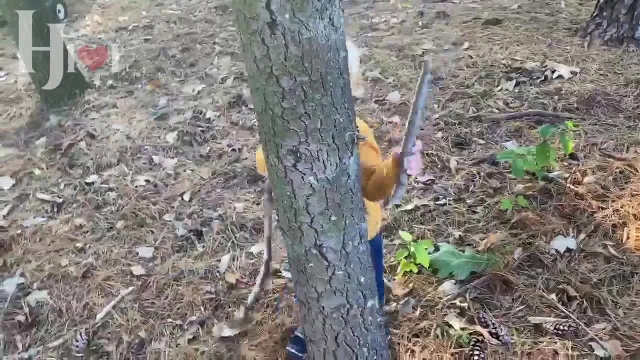 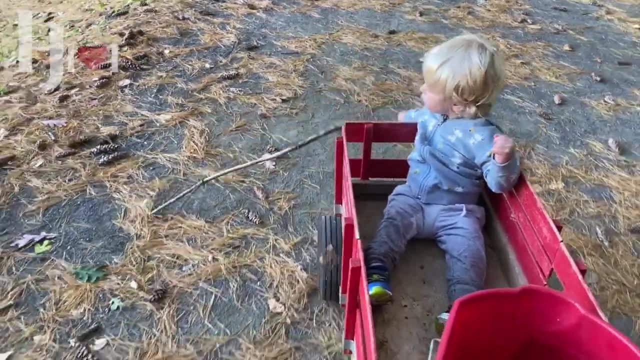 The other thing is when you're out on your nature walk- and you're seeing, Here I have a wagon. Wagons are great for nature walks, for toddlers And strollers are too, But you can get in and out of the wagon and you can put your treasures in the wagon. 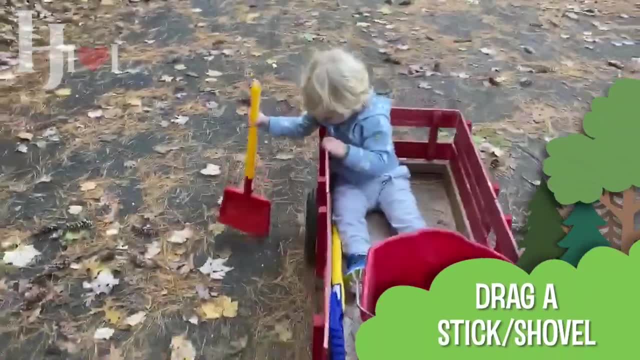 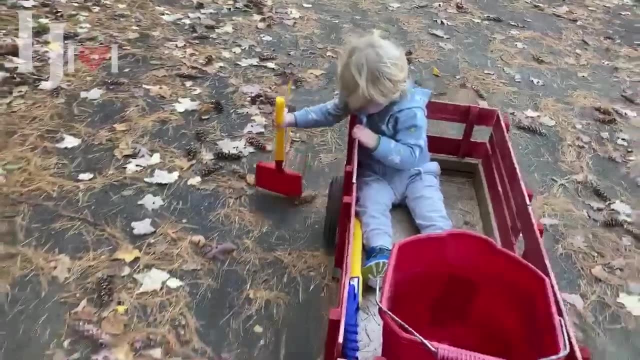 But in between times, there's something that my children have just done for hours is to drag a shovel or to drag a stick behind them, And there's so many interesting things happening And you probably you may have to show them how to get started on this. 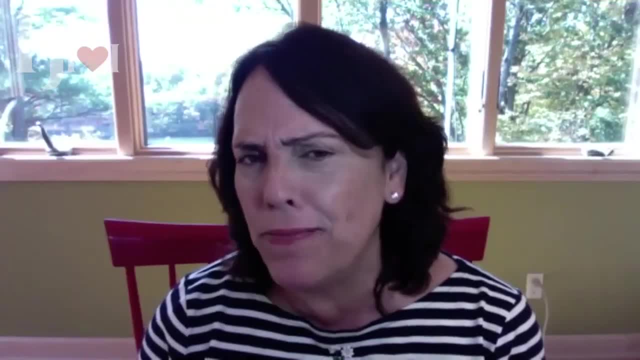 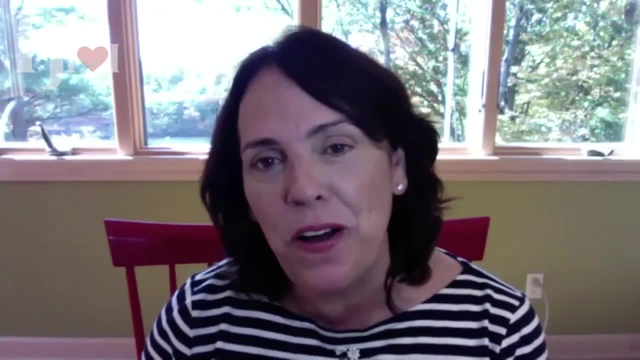 But even at a very young age they can do this. So it makes this great sound, It makes this vibration, It makes a mark in the dirt or the sand which they can look back at and get that sort of object permanence thing or that sense of how far they've come. 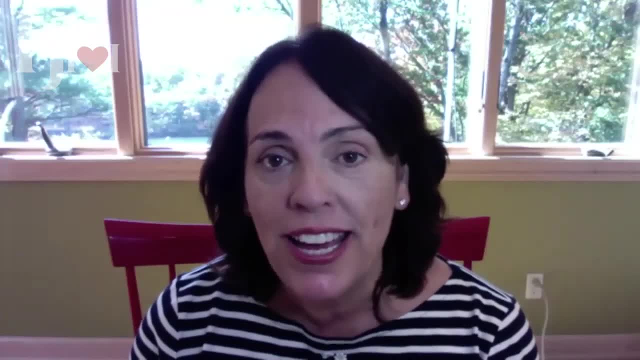 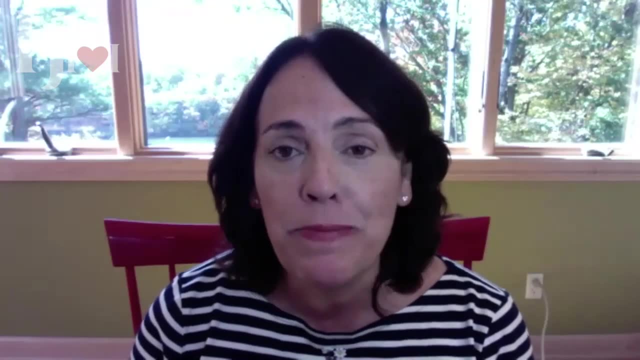 How far they're going, That they just really enjoy. Sometimes they'll even get to the realize that picking it up and putting it down makes a pattern or sort of makes a musical sound. But this is something a lot of kids will do for hours. 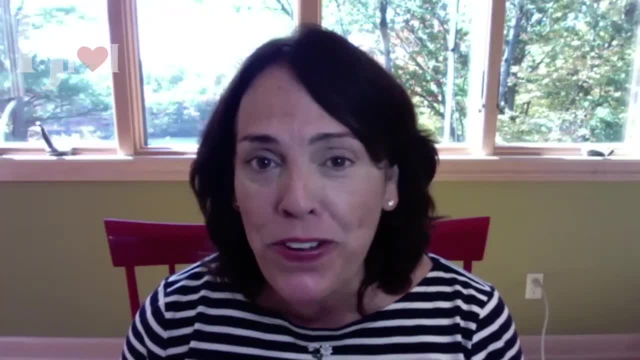 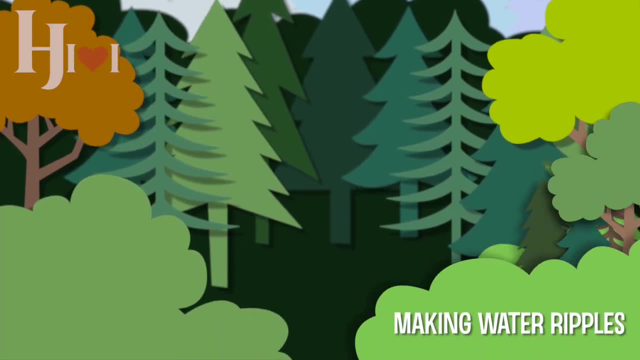 Do it over and over again And so again, it's joyful, It helps them learn something And you can get a longer walk in, because they'll just keep going on this for a long time. Another thing is if you can find a still body of water and the right size stick to help your child just 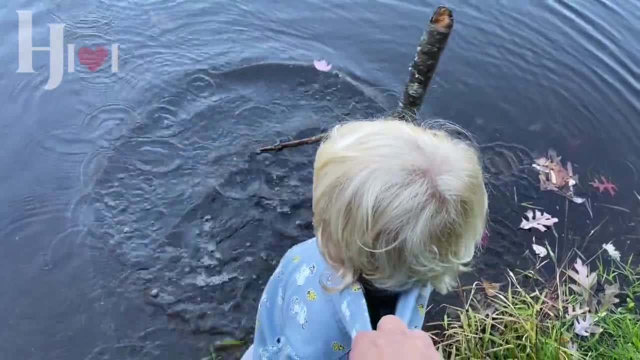 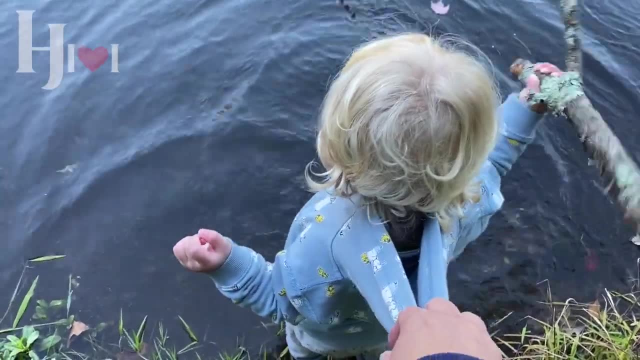 Have this experience of making these ripples in the water. It's a great way to look at that cause and effect. It's beautiful. Again, they get that idea of I'm making things happen out here. You can take it out, You can take it in. 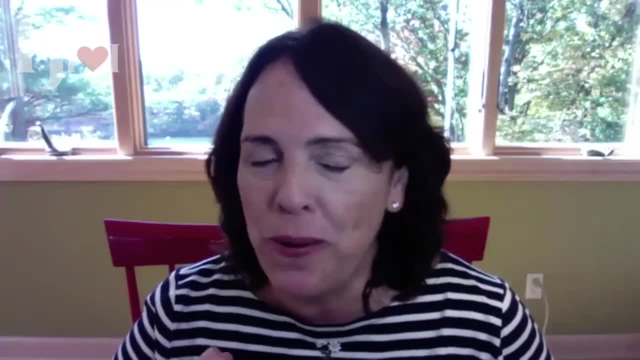 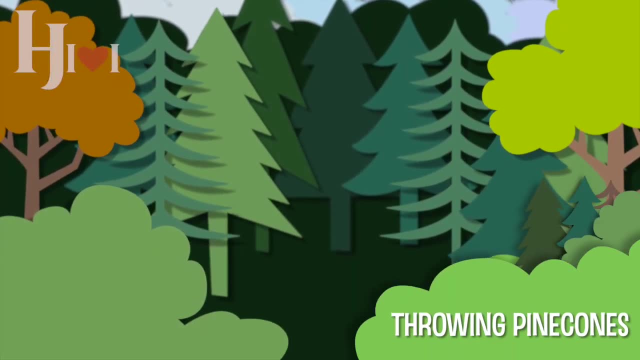 You can figure out yourself how. you know, small or large amount of pressure can make different things happen. Kids, toddlers at this age just love this. Okay, Another great activity is taking pine cones and collect them in your bucket. So of course, that's an you know. 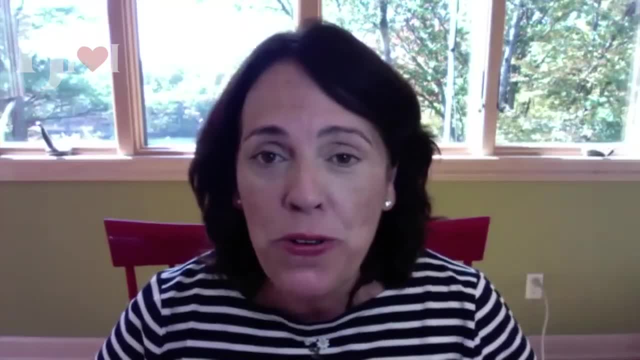 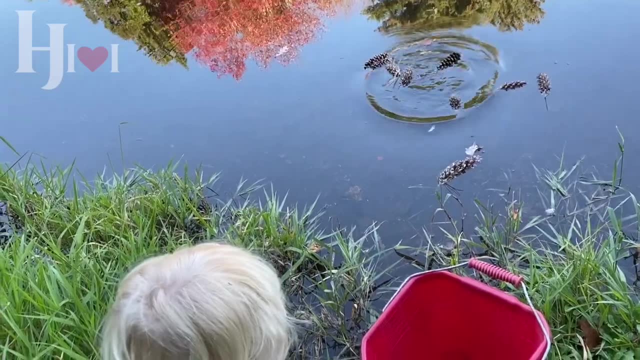 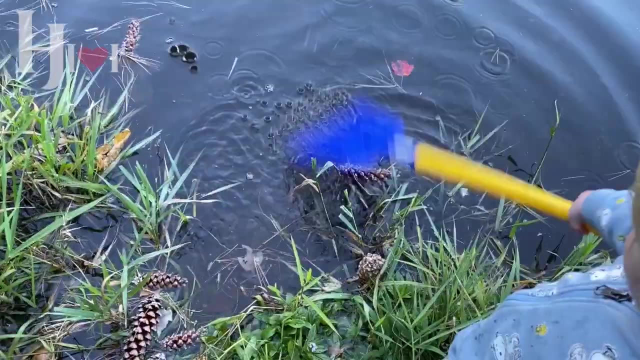 that's an activity in itself. And to throw these pine cones into the water And of course they're going to float right. So this is very different than rocks: They float And this is a very enjoyable exercise. But the next piece is to have your child's handy rake along and to take the rake and pull them back. 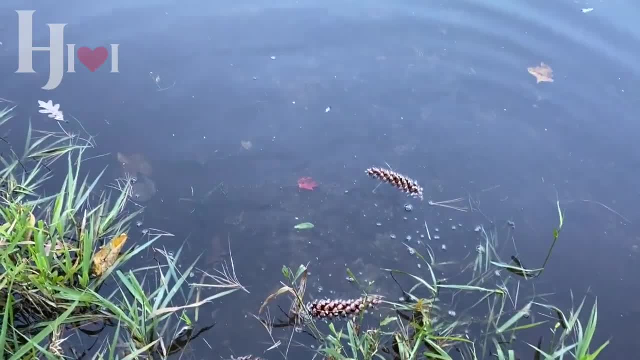 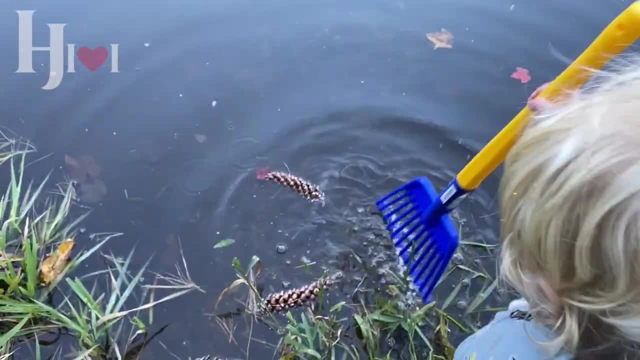 And virtually every toddler, the first time you do this, will just laugh delightedly: My look, I did too, Because they're so surprised that you can just pull them back like that. right, This is a fantastic experience for them to throw them back and pull them back towards them with the rake. 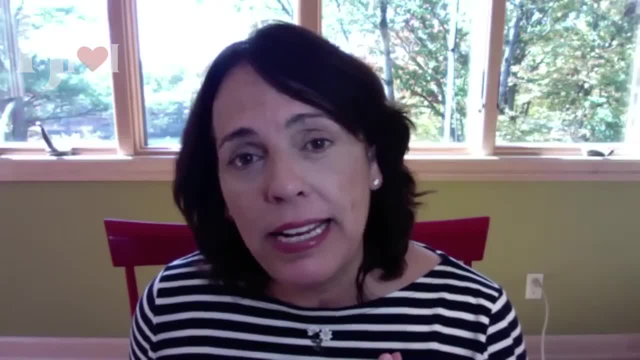 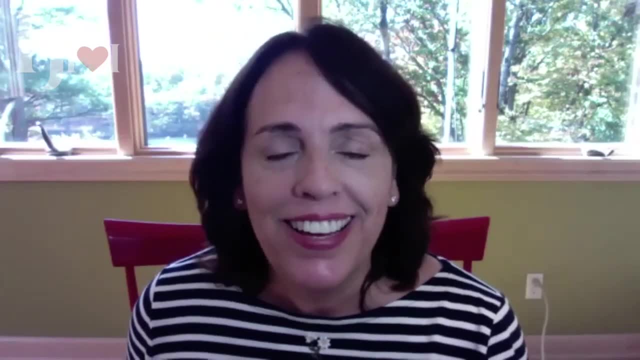 They also can probably be- you know, as long as they're 18 months or older- get the idea that if they just sort of hit the water they can make little waves that will also bring that pine cone back. So this is a very enjoyable experience. 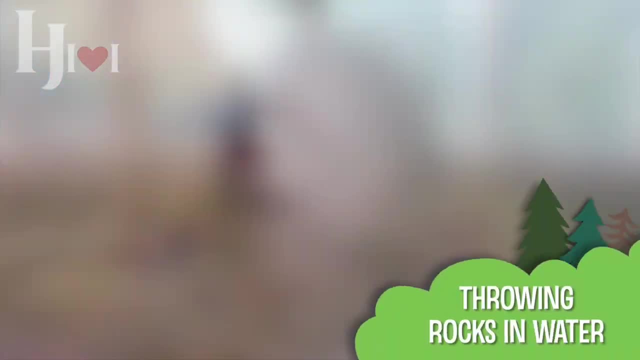 The next thing that kind of goes with that is throwing rocks in the water. So this is a completely different experience, right, And you know you can do this where you put them in a bucket, You can have a little net bag. 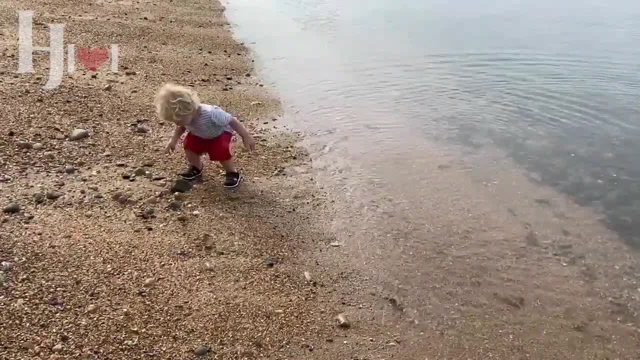 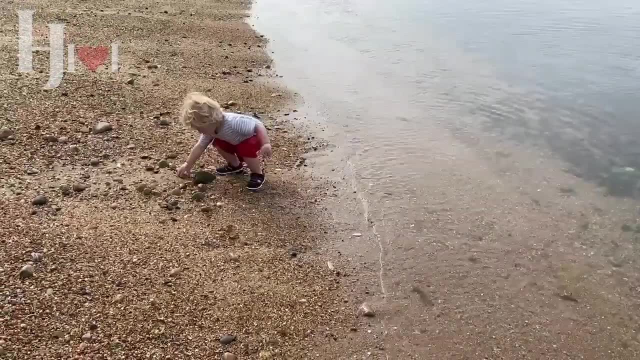 Whatever you want to do so that you've got some rocks to throw in the water. Of course, if you're on a beach with rocks, it's- you know- all the better. But again, they can have that experience of throwing it in the water, possibly bringing it back, or possibly not. 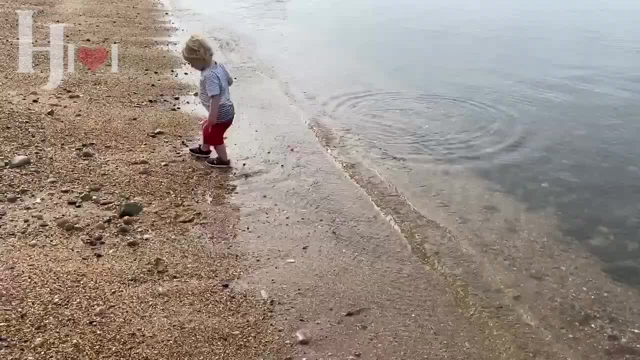 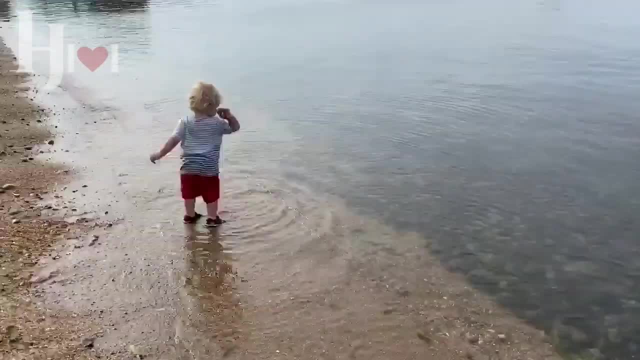 It depends how deep your water is. But that goes along with that big idea of what sinks and what floats, And so then you can see back here in his high chair just the simplest experience at home where we brought some of these back, And he can see these plastic containers are so great. 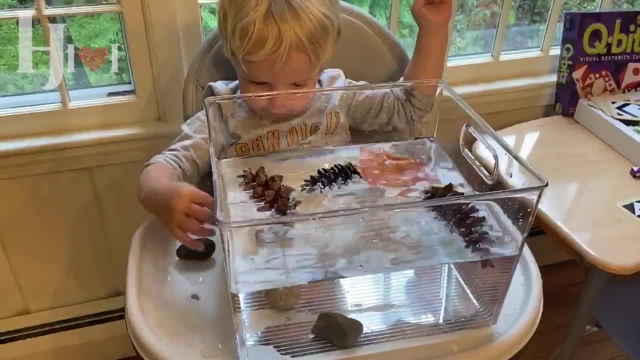 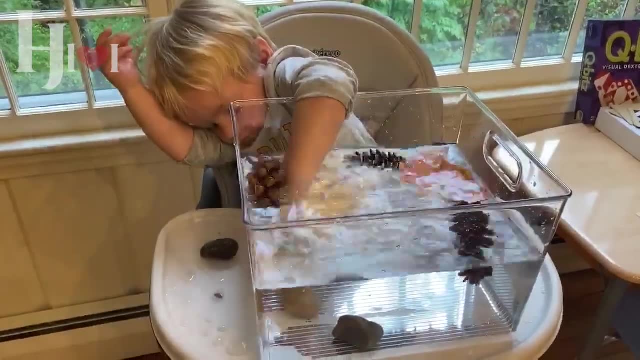 It's M-design made in USA, But he can just look through here and he can see- oh yeah, I remember this right, Pine cones, float rocks, sink, And you know you can give them a variety of other ideas. you know different things that they can experiment once they get home with that. 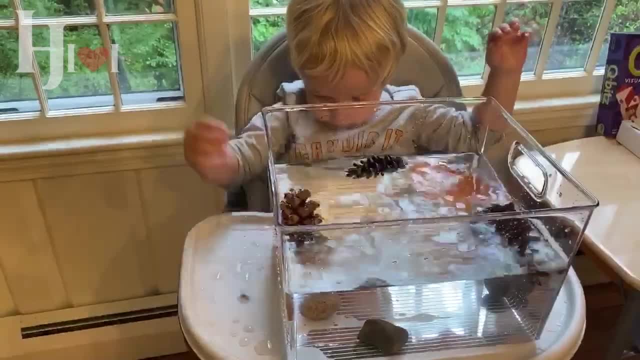 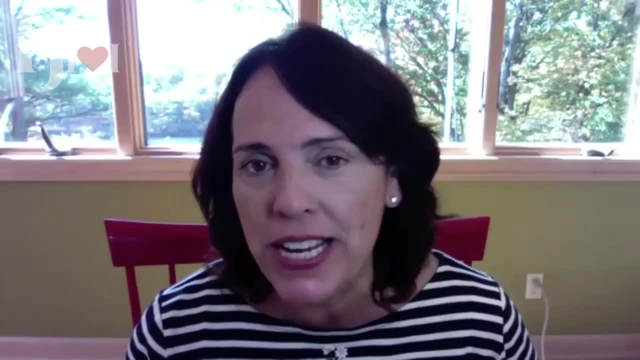 But that's something that keeps going. But having the experience in nature, the experience when you're out there in the big world, I think really makes the float and sink at home much more intriguing. right Gives it a lot more context and depth. 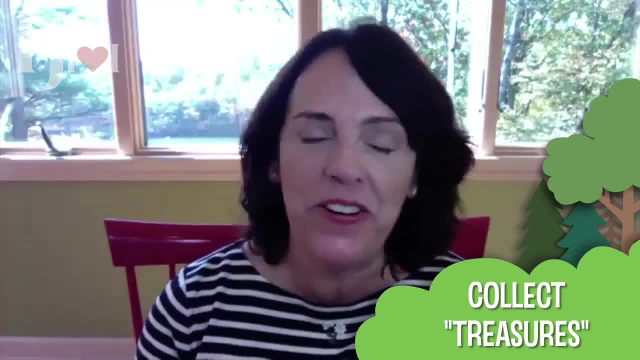 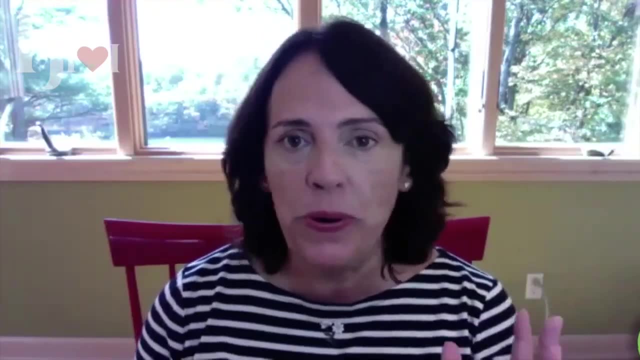 So another great activity to keep Keep kids engaged when you're out there on your nature hikes is the idea that they can take, they can see something and they can put it in the wagon or the stroller or you know if you want to carry the bucket. 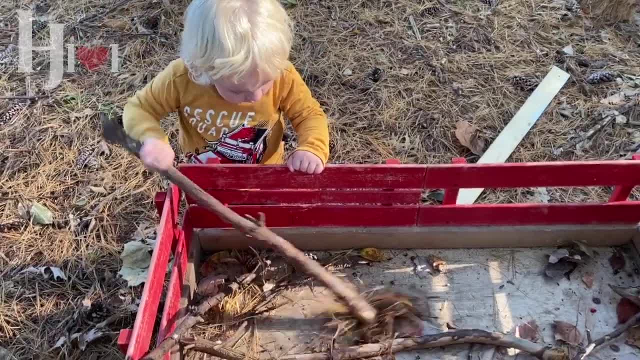 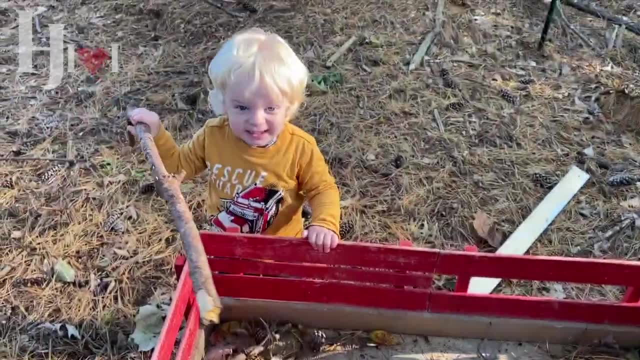 We have this handy, dandy, made in USA bucket with us And you know, having the bucket with you means that they know they can always do this right. So if they see a pine cone, if they see a stick, whatever they see they can put in there. 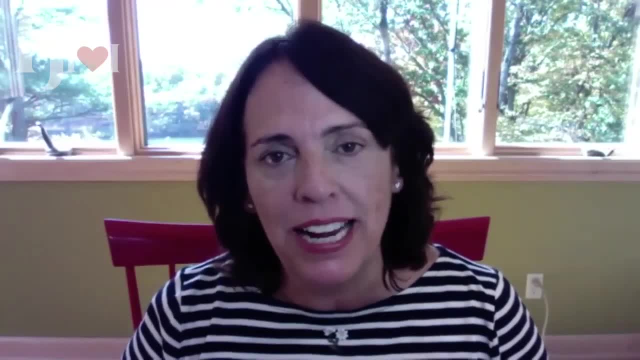 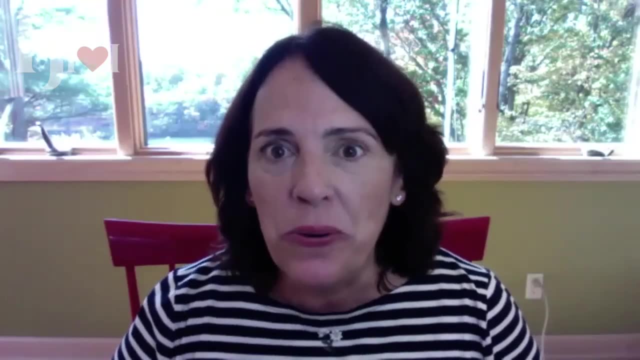 And the other thing is, by having it in the wagon it sort of reframes that right And instead of just this whole big world of nature, they can really look at things differently. They can look at things a little more closely and start to appreciate the glory of this world that we live in, right? 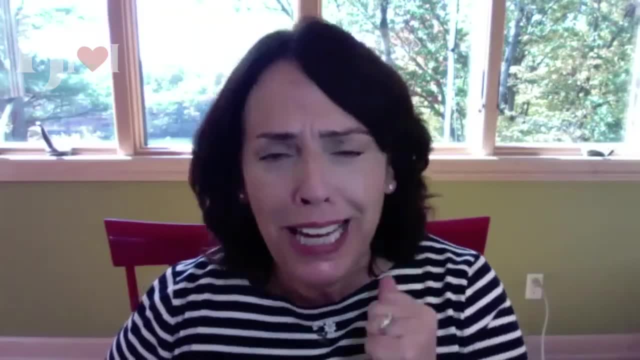 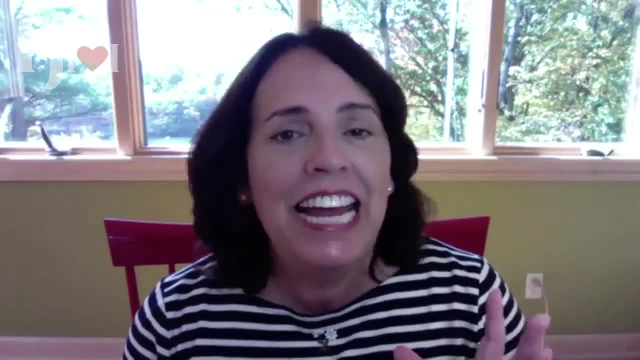 The amazing intricacy of it. You know, sometimes they're going to want to stir things up in the wagon. They're going to want to, you know, put all kinds of different things that they find in there, And it's not always what you think is interesting. 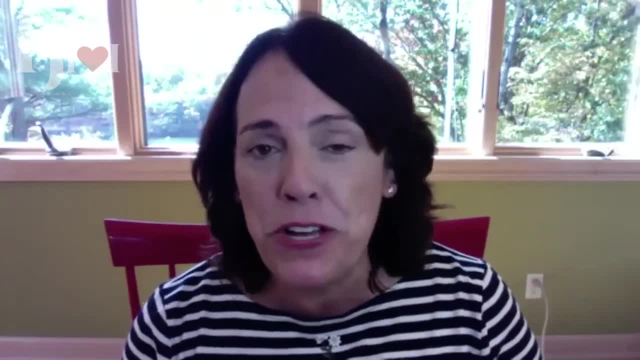 But as long as it's safe and it's great for you to, ahead of time, you know, know, like you know, make sure you know what poison ivy is or whatever, Like you're not going to have your child pick that up. 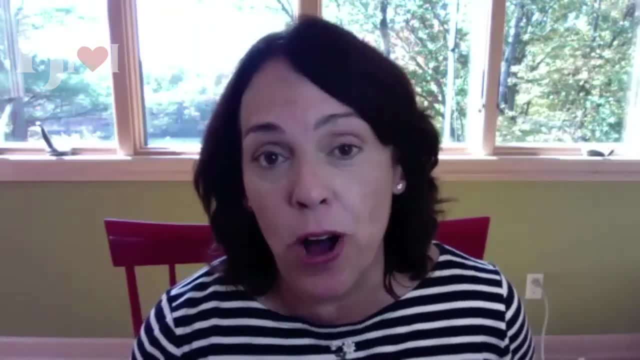 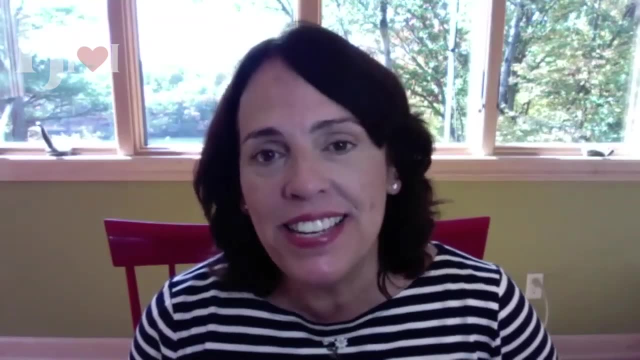 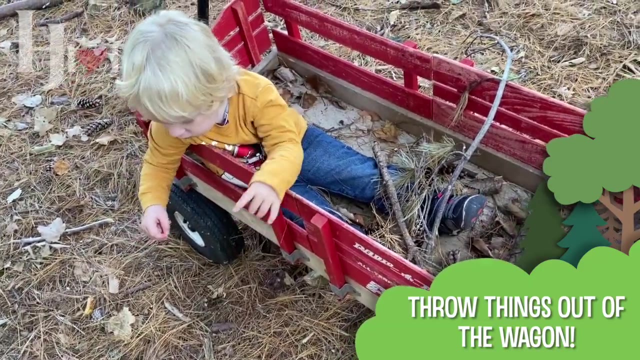 Sitting in the wagon- they're with it Also can make the walk go longer. right, Because they've got something up close to do. But intriguingly, I have noticed that toddlers find it even more enthralling when you know you give the signal that it's okay now to start throwing things out. 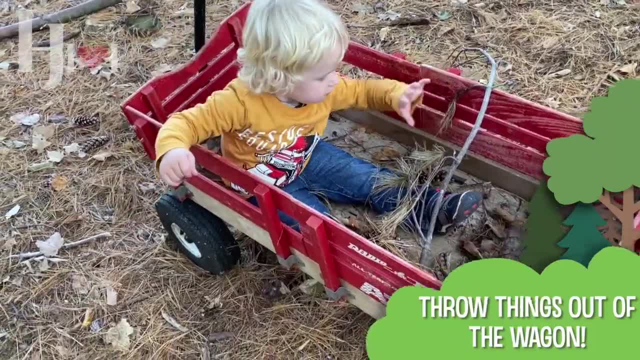 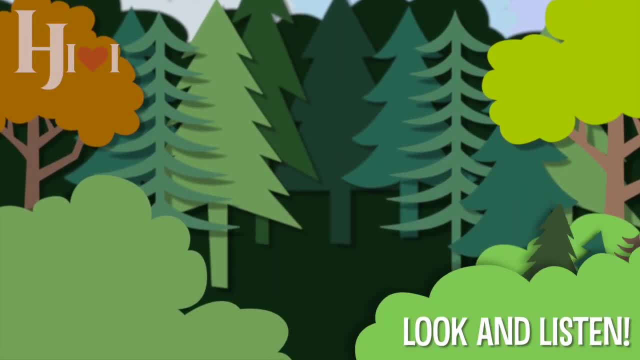 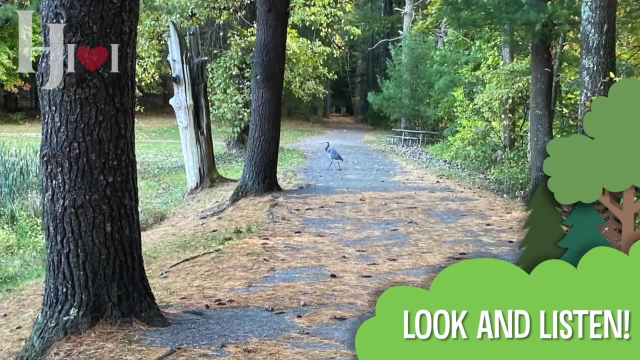 And I have found that my toddlers love to just one thing at a time: throw the things out- And this seems to be a really powerful thing- to throw it out of the wagon too. So the next one might be pretty obvious When you're out in nature- and you can see here that we just were on this nature walk and this beautiful heron was just standing in the middle of the nature path. 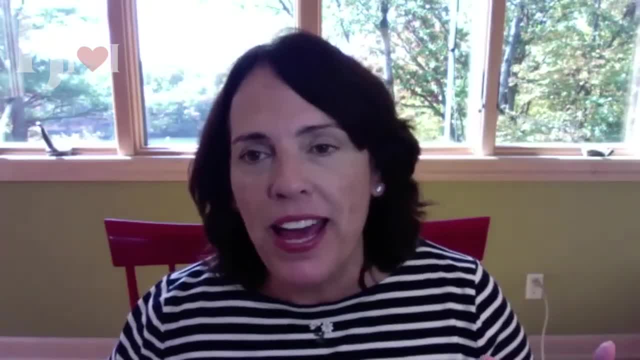 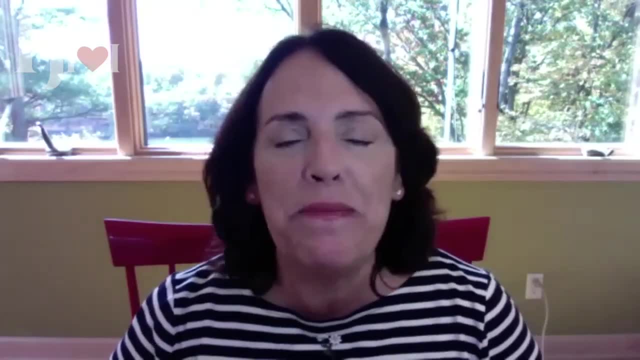 You couldn't believe it, It didn't want to leave. Eventually it flew away. These kind of beautiful moments where you take notice of them and you act excited about it when you're out there, is going to make your child a lot more excited. 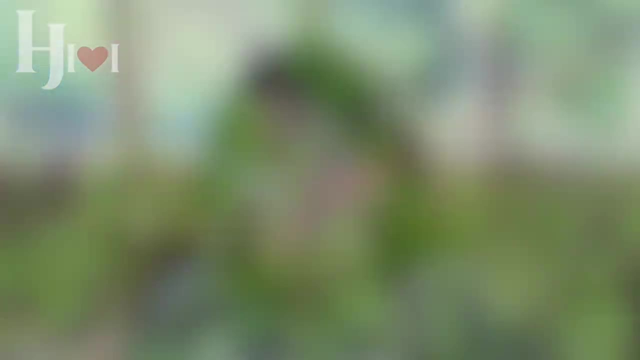 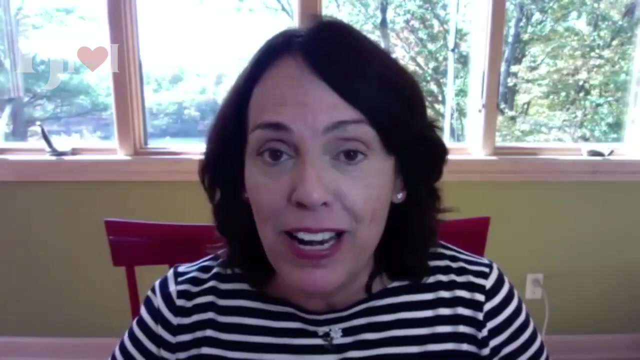 Whether it's a squirrel or in this case you can see this picture. we saw a walking stick blended in pretty well with the pine needles on this boxwood To take that time right to act, excited about it and show just like a. you know you want to model that you love reading, so your children love reading. 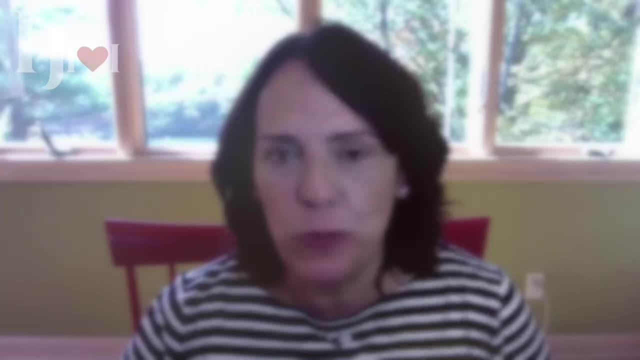 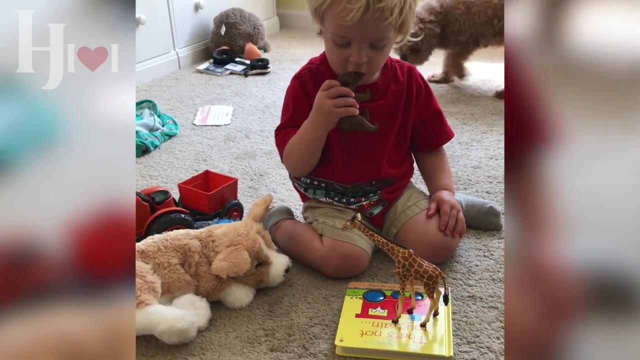 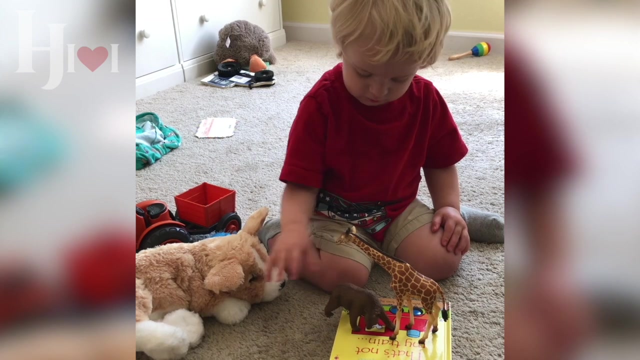 To model that you appreciate the glory of this world can really help that toddler realize, wow, this is it, This is amazing. And when they go home to play with it, You know, even if you don't have the exact same plastic animals, to have that experience of playing with what you did and thinking about it again is one of these things that's really building on your child's understanding. 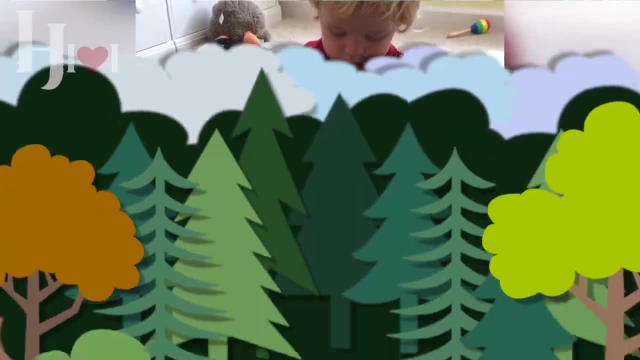 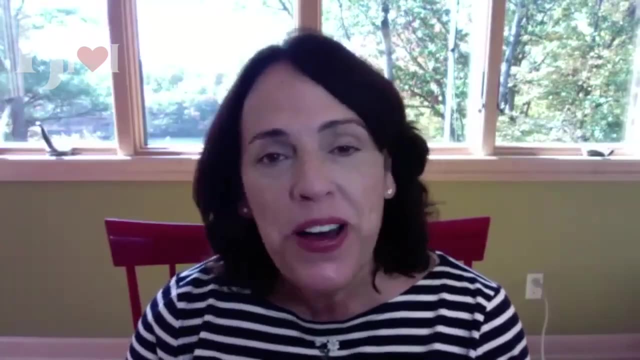 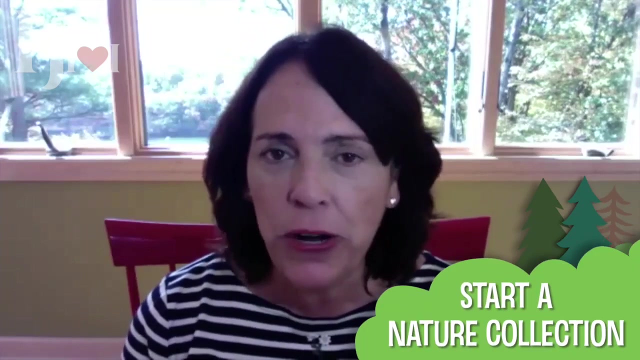 Of nature, The world And the processes that are in it. So, even though your child probably found it very therapeutic to throw the things out of the wagon that they had collected, having your child be working on some kind of collection at home somehow is something that a lot of toddlers just really enjoy. 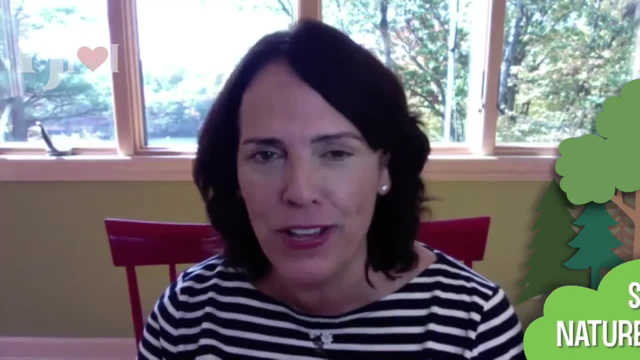 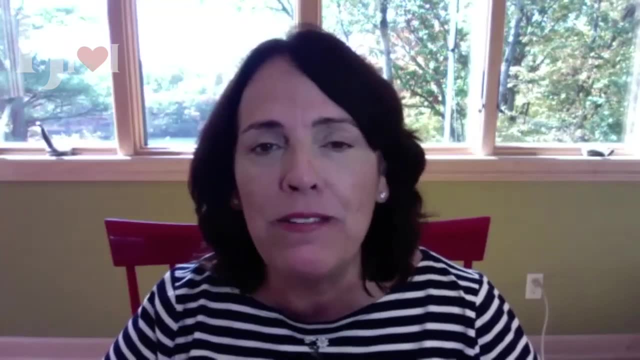 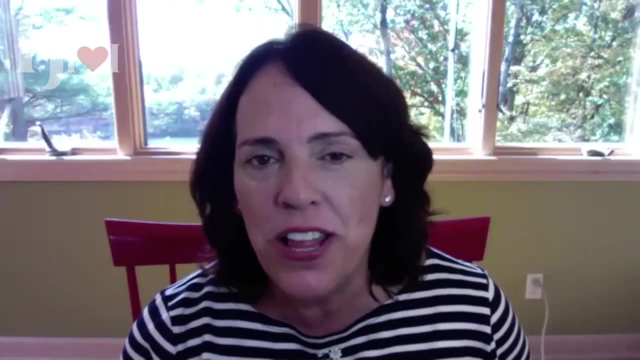 That feeling like, hey, I know that happened because I have this rock from there. So, just like I guess you know you're out in nature Museum or your art museum and people want to buy something from the gift shop. Having something that your child is interested in and letting them start building on that might be really great. 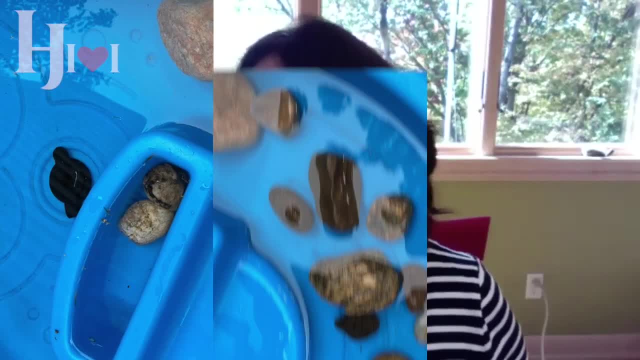 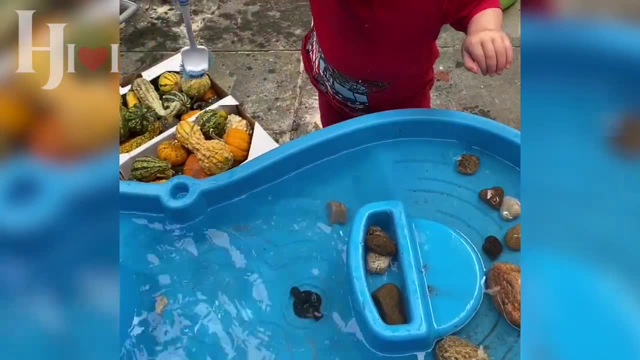 So it could be that you take a little stick every time and they're going to build up sticks. My kids have really liked rocks, So you can see here that once he has the rocks home, we wash them in the water table And then there's all kinds of different ways to display them. 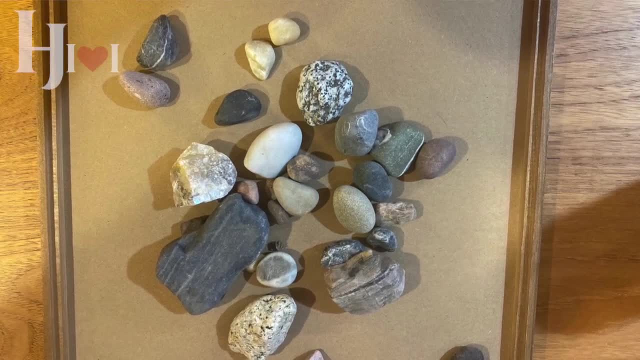 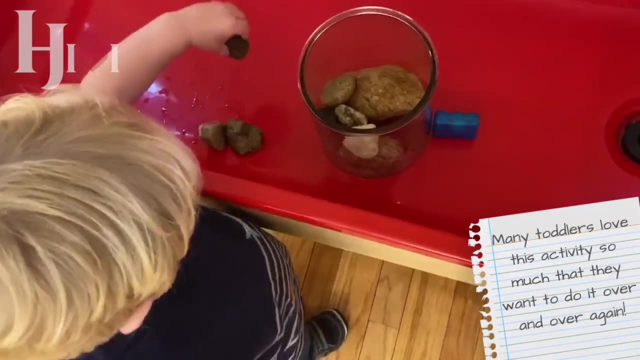 And the nice thing about this is your child can really do it, right. This is something that your child really can: put rocks in different containers And you put it up and you're like, wow, you made that collection for us And it's not like you did part of it for them, right. 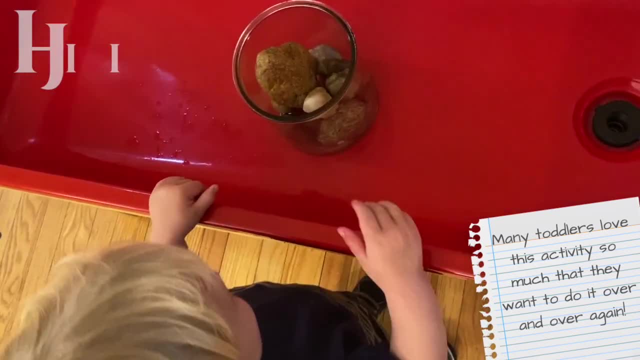 They really found the rocks. They can really wash the rocks When they're very young. pretty much as soon as they can walk they can put them in a jar and you can talk about how they did it. It's very enjoyable for them too. 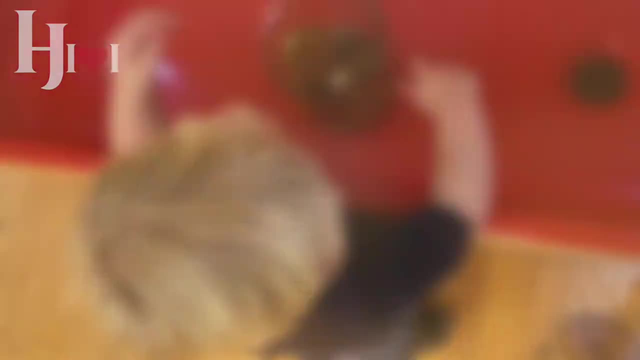 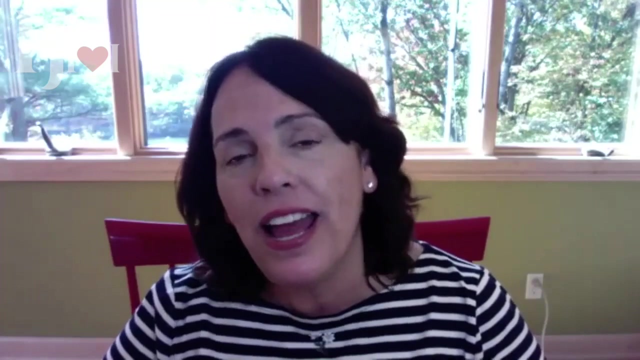 But also they can start to notice big little different colors. There's so many different kinds of grouping and sorting that you can do, And you wouldn't have to do rocks. This is just an idea, So that every time you're out, they're also looking for something right. 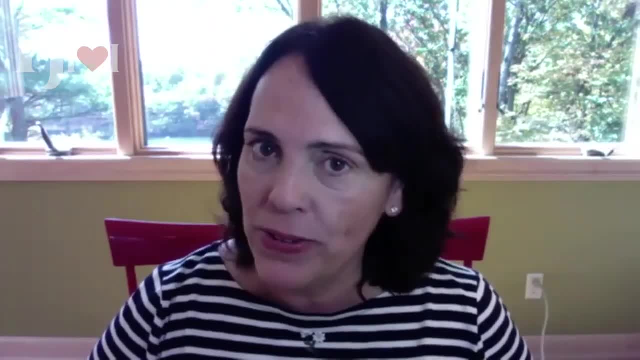 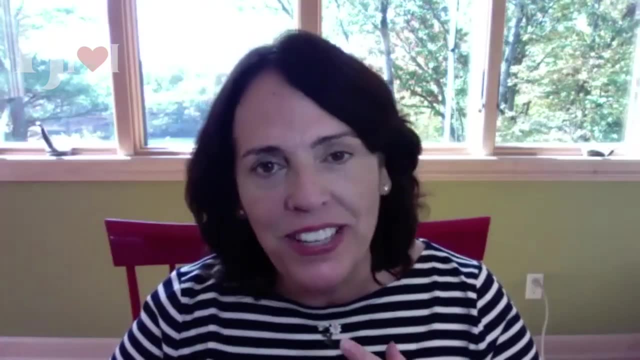 They're thinking to themselves like, oh hey, there's a rock. And it's part of helping that brain development to notice details, notice what's going on and be involved interactively in this process of noticing, enjoying and loving the beautiful outdoors. 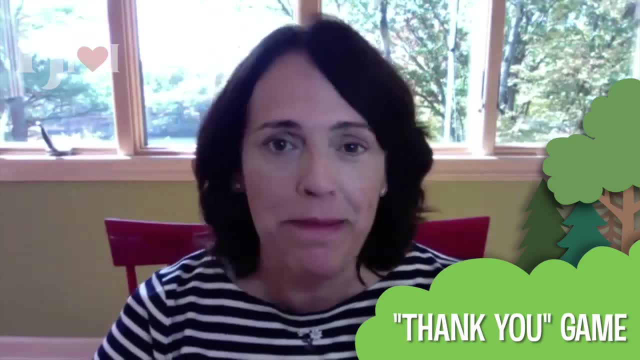 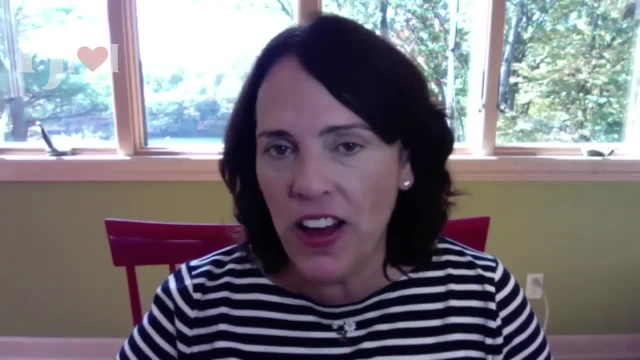 Okay. So this next thing I call the thank you game, And this is something I've done with my toddlers with great success. Basically, it's very simple. They help you find some things that you're going to put in some kind of lightweight tote that they can easily- you know- maneuver or carry if they want to. 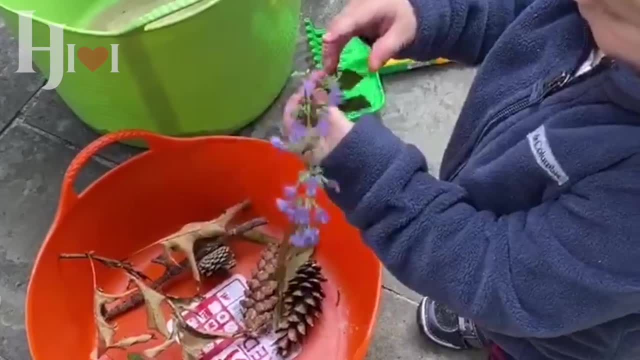 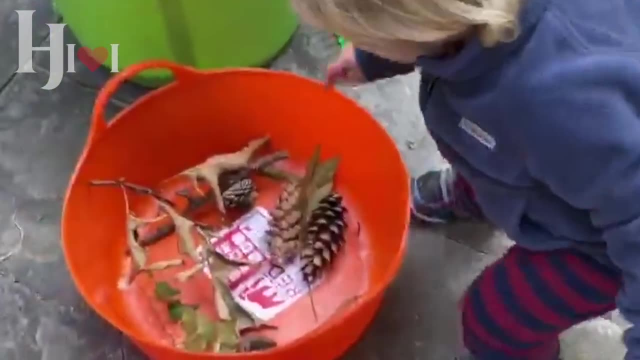 And then you sit down and you have this very you know moment of looking them in the eye and noticing them. You're not on your phone, You know you're not like talking to somebody else And you just tell them: hey, let's play the thank you game. 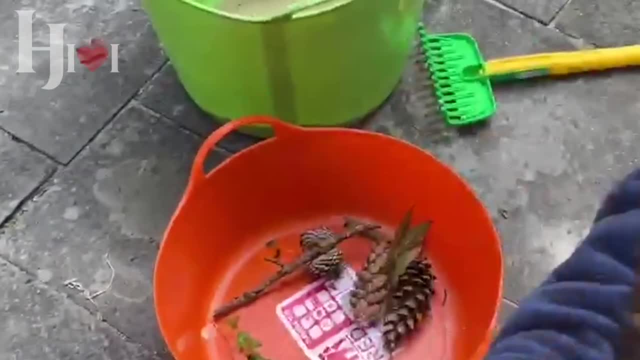 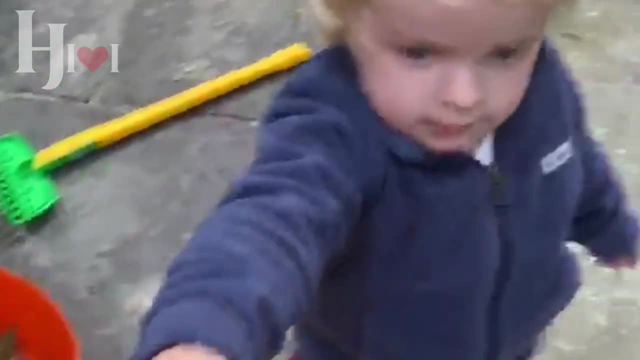 And then they will learn to hand you each of these items, And then all I do is say: oh, thank you. But I notice something about each of the items. It could be the color, It could be the prickliness of something. 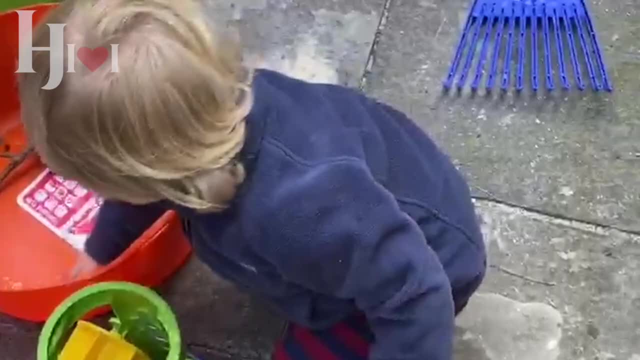 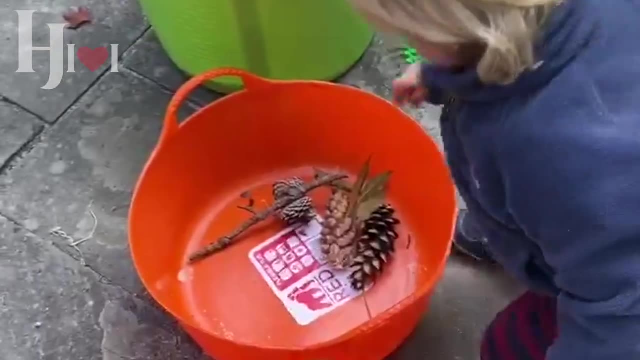 It could be any kind of thing that you want, But what I'm doing is not just working on language skills, which happens- but I'm also helping that child to notice things more carefully. right the details involved in each of these things. 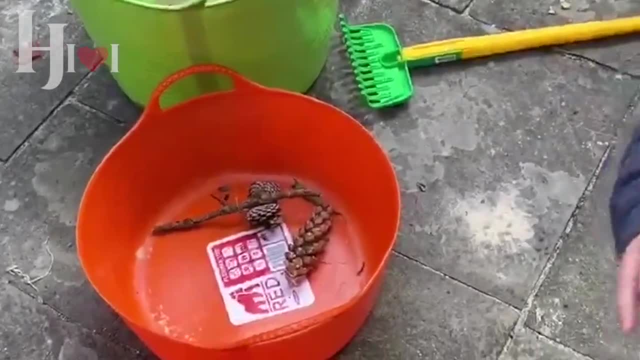 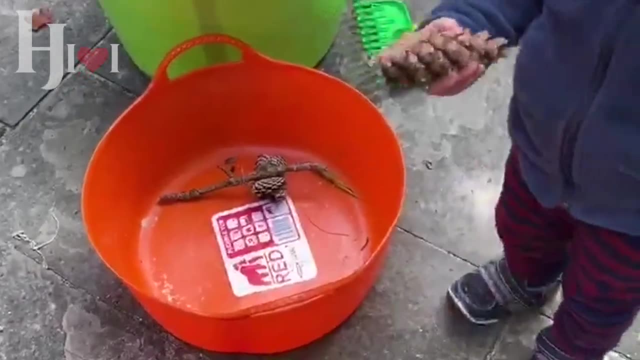 It also just seems to be super therapeutic for them to be doing something where you're just saying thank you back and forth- And I guess part of it is. I really say thank you big with each thing And I let my facial expressions show that. 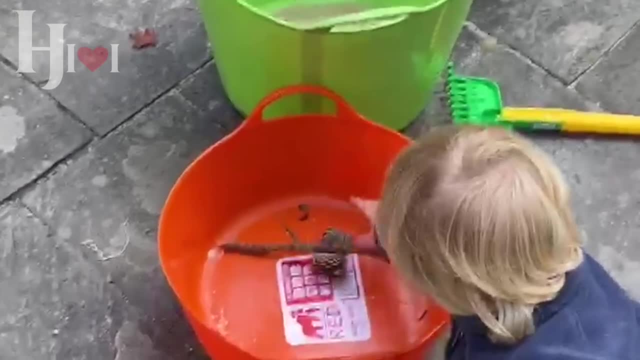 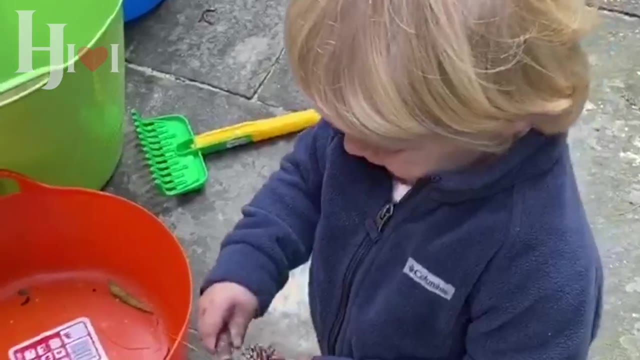 I'm looking the child in the eye, I'm engaged in seeing and saying thank you, You did this thing for me. You're giving me this gift of nature. I've had kids do this for a long, long time. Toddlers seem to be particularly loving this. 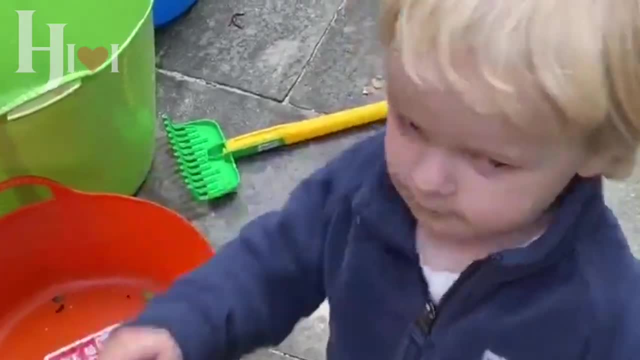 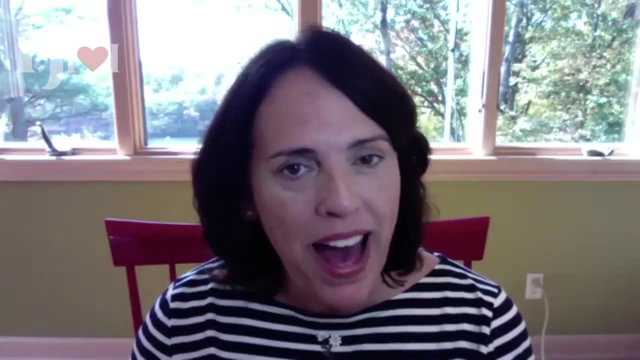 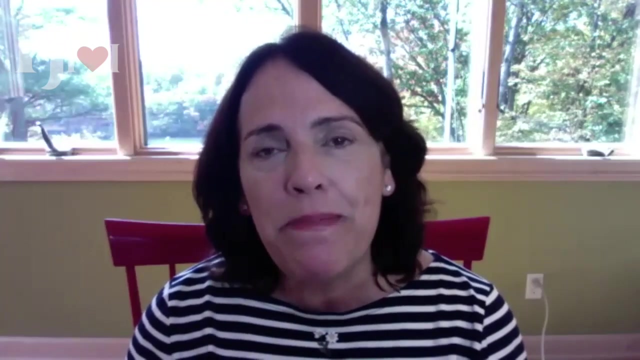 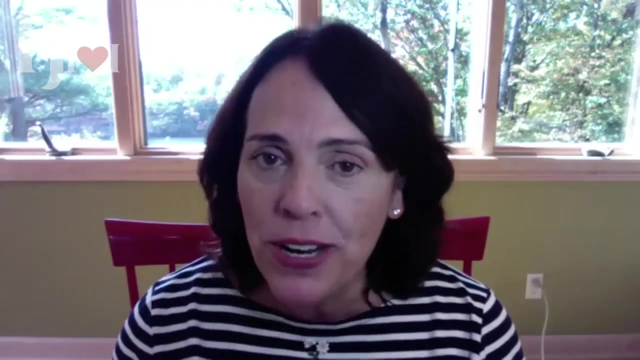 And as your toddler gets older, what you say about each thing can get more and more complicated. I know it seems really simple, But this is something that I feel That, when I look back on, was not only just almost wholly bonding kind of experience with my children, but something that I feel like I started to realize who they were as an individual, who they were as a person, based on what they wanted to say about each thing or, even before they're talking, what they wanted to show me and point out. 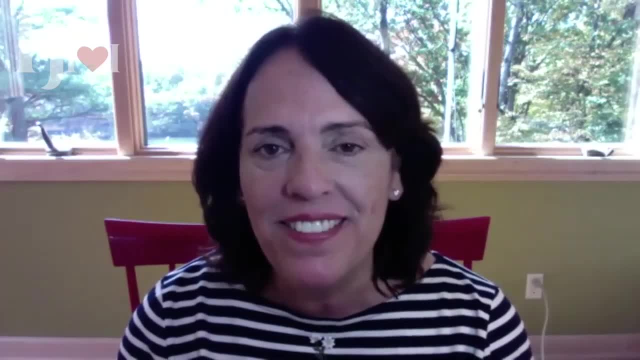 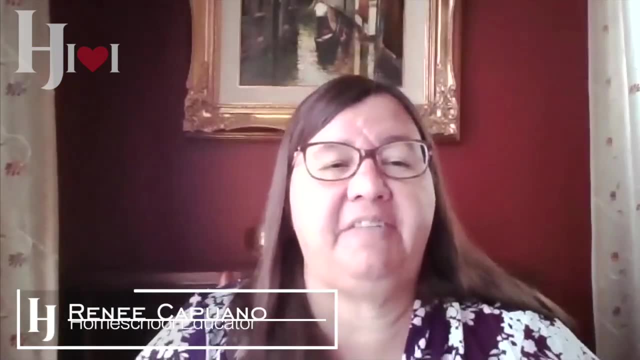 So I don't know. I hope that you might enjoy it as much as we have. What do you think about all this? I really think this is really wonderful. These are such great activities for your toddler, for you to be out enjoying nature together. 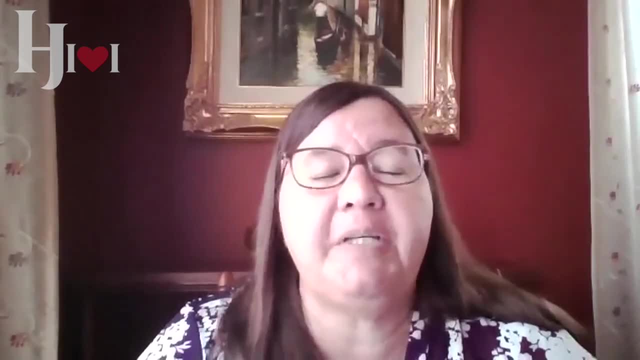 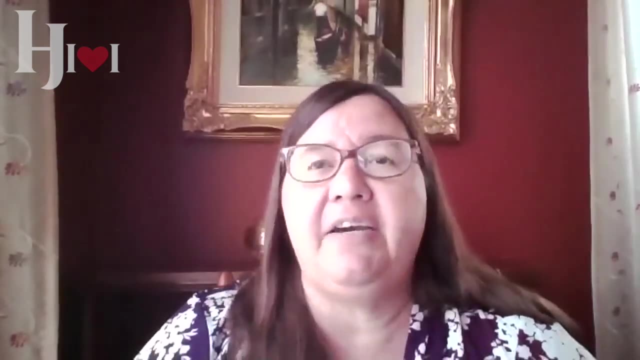 You're having fun And you're also building those brain skills And you're making those connections And I really love the thank you game. That is such an opportunity. As Helen, as you said, you're not doing other things, You're very engaged with your child. 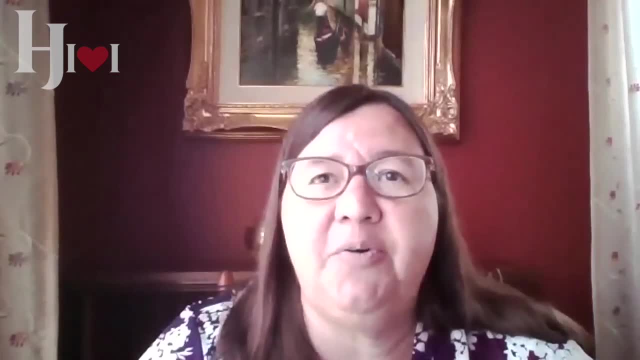 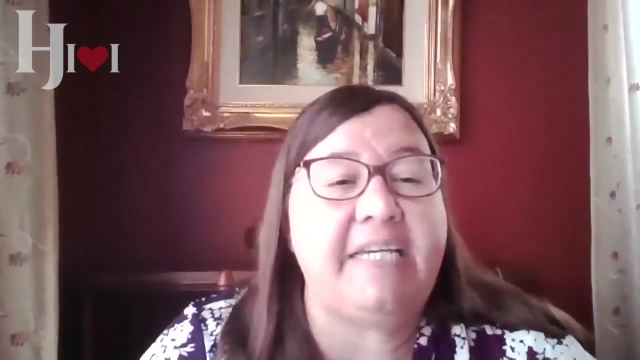 You're very focused And saying thank you And noticing that little detail. It builds up this expectation, even in a toddler, that you're noticing what they're doing And you're appreciating what they're doing, What they're showing to you. 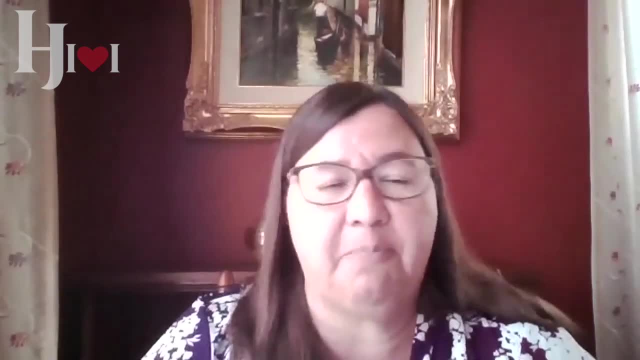 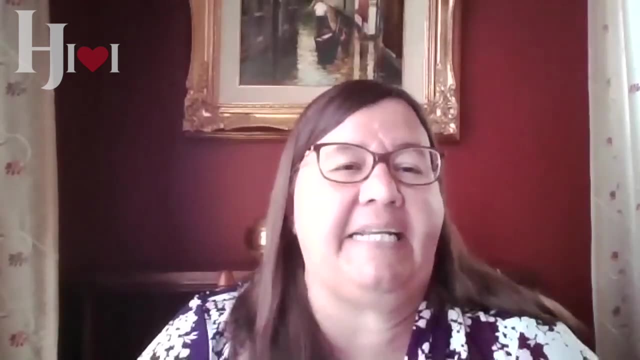 And it's not just a thank you and move on, But it's a thank you. Look at how prickly this is, Or look at what a bright orange color this is. It is also instilling in them that there's something different and unique or something valuable about what they're doing. 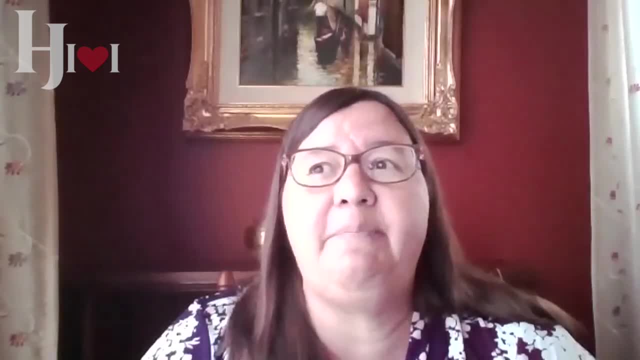 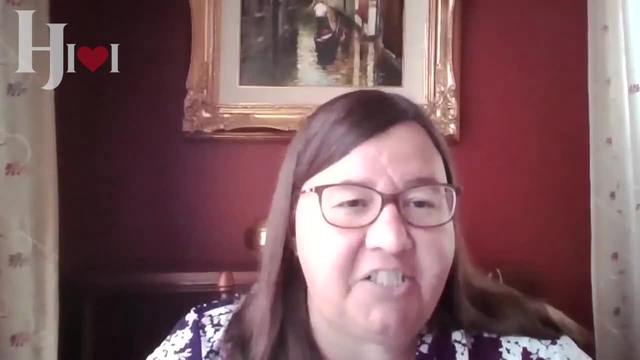 The objects that they're picking up, And it makes it so much more fun that you're noticing those things. It's not just the fun of picking it up and handing it to you and putting it in the wagon, But it is that you're engaged and you're noticing the world around you too. 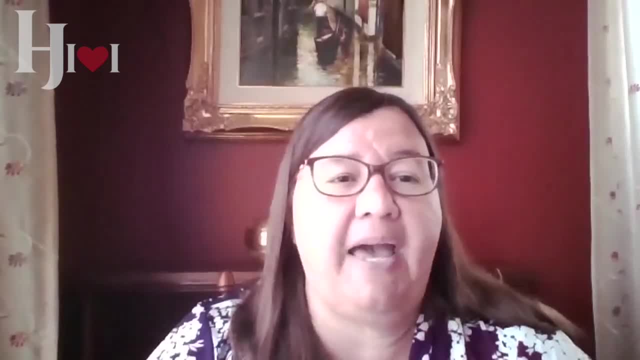 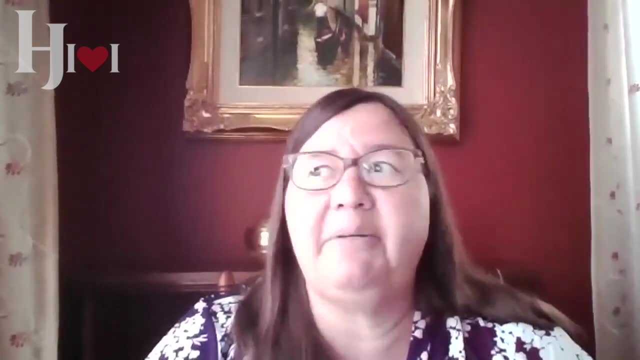 And that teaches your toddler the value that you have in what they're doing And the value that you have in the entire activity. And I really love that Because it builds so many skills And it builds, as you said, that bond between you and your child. 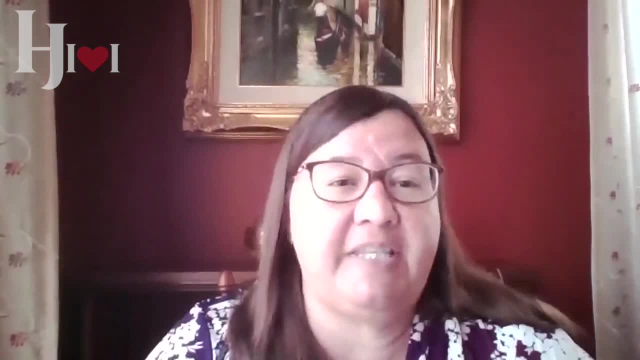 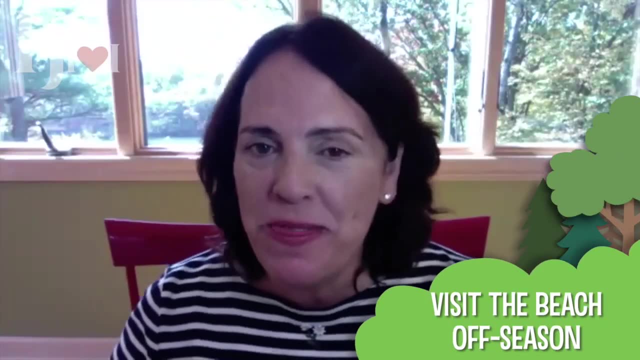 That they can expect that you're going to value the things that they're valuing. Thanks Helen, Thanks Renee, Because the good thing is just don't forget the beach, Particularly if you're a person who burns easily, You might actually enjoy the beach. 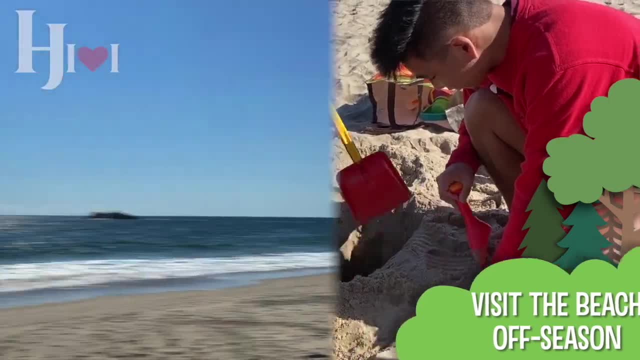 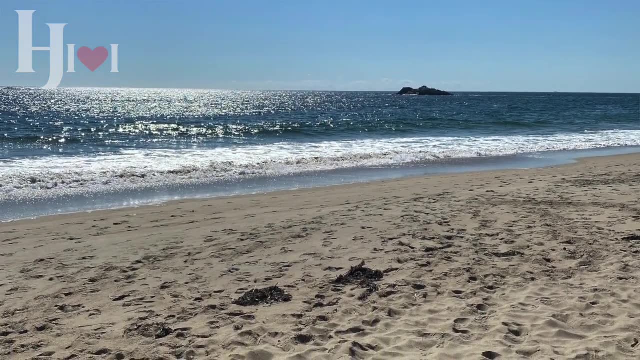 Your child might actually enjoy the beach more when it's not hot, But, as you can see from these pictures, invariably wherever I've lived, just like, nobody is on the beach after August, But you know, you've still got the fall, the winter and the spring to enjoy the beach. 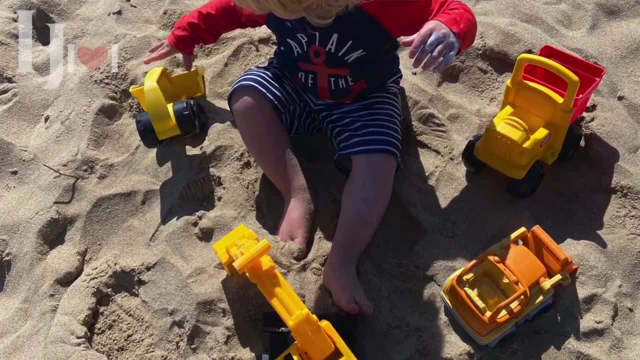 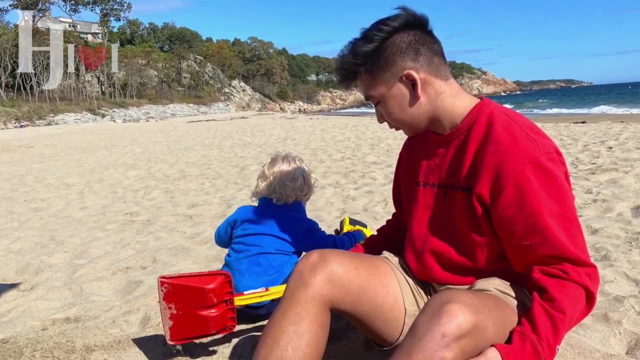 Sometimes there's like literally no one else on the beach. This is actually a public beach. There's nobody here at all, And of course you probably don't want your child to go into the water when it's getting colder. But there's so many great things you can do if you just remember to bring things. 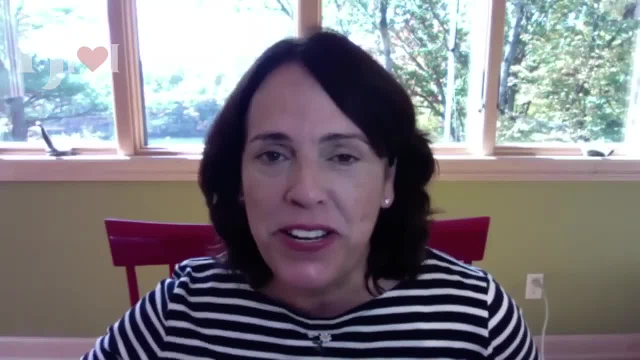 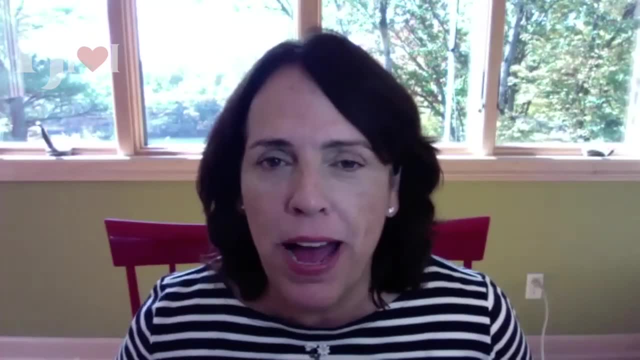 So bring a lot of trucks, Or bring- like my son is here on this particular day too, Bring a good sturdy shovel that they can actually dig in. I've had these Several times, But having a set of tools for your child. 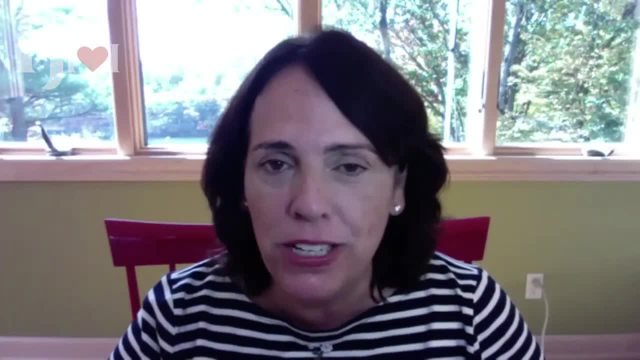 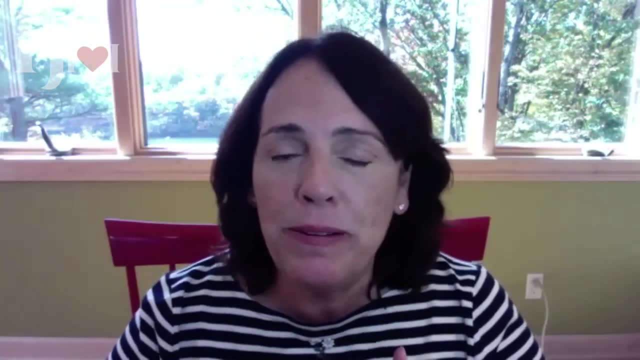 So a rake and some shovels that are really pretty sturdy. These are made in Germany, Not actually made in the USA, But they're very good. The way that they're connected is they're going to break. It really helps them to be able to do a lot of things. 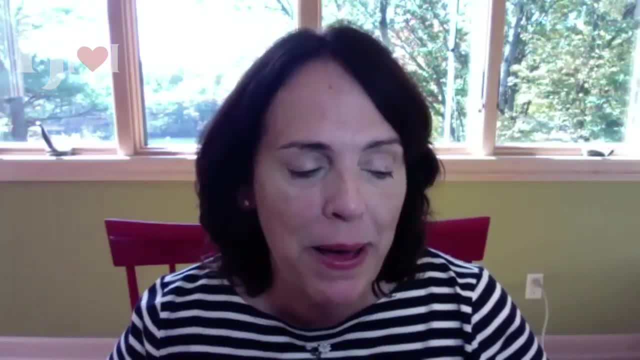 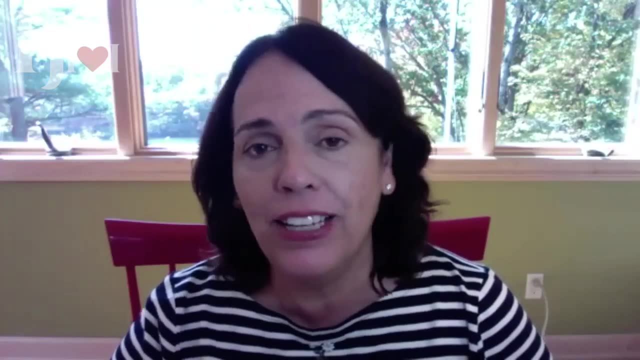 Like to dig a deep hole To, you know, push over a log, It's a strong enough thing to happen. So, anyway, that's just a thing to think about. Like is there still the beach that I could go to, even though it's not? 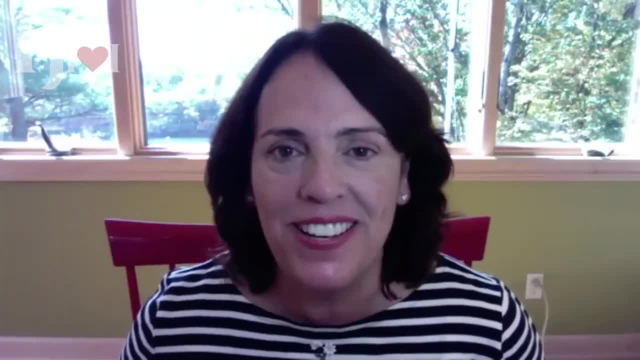 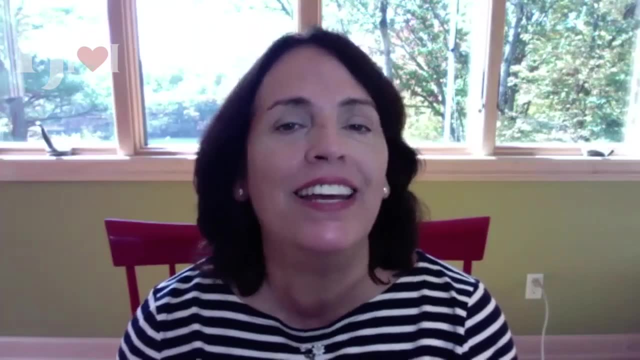 I've taken children in their snowsuits to the beach And they've had a lovely time over and over again. So the other thing is the beach is a great place to play pretend, Especially when there's not so many people over. So you can see that he's like crawling delightedly. 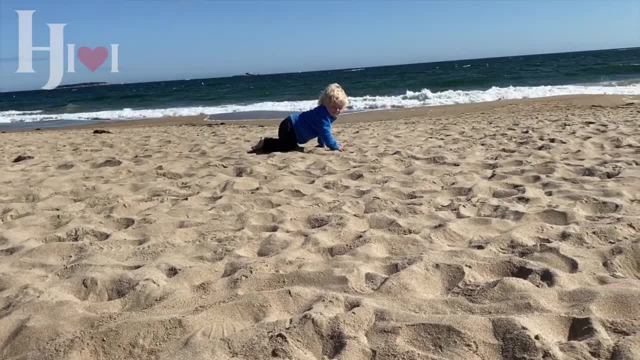 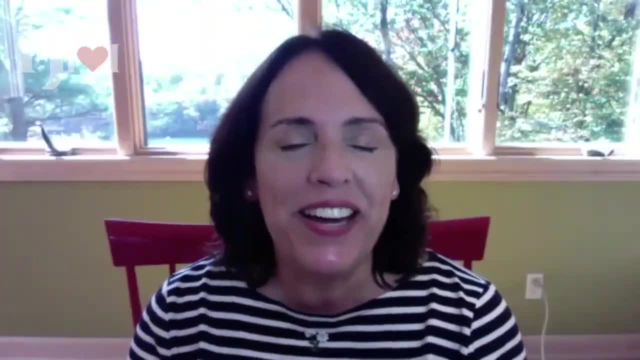 He's pretending to be different animals on the beach, Making animal sounds, And he can crawl around. It's not going to hurt at all, But it's very interesting And it's very tactile. So, anyway, these are two things that I find that work very well. 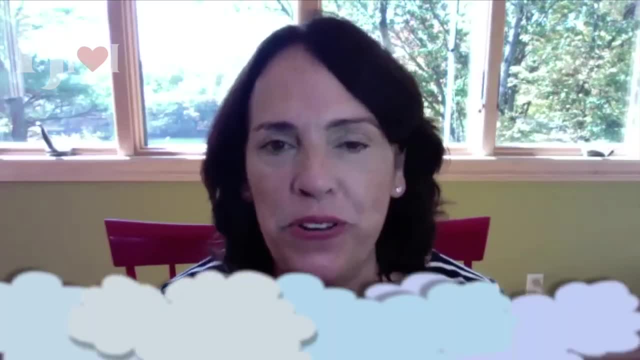 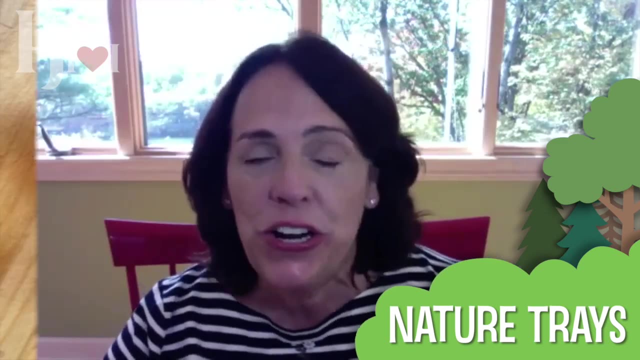 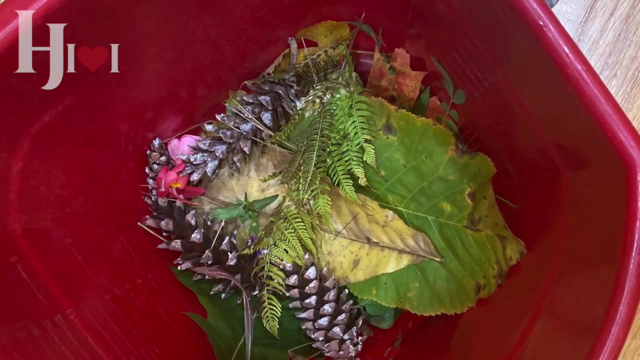 Even in the off season, To enjoy the beautiful ocean. So the next thing I'm going to call nature trays, And this is the idea that when you're out in nature, you've got your handy bucket or whatever you do, And you are collecting things sometimes that you're going to take home and do different things with. 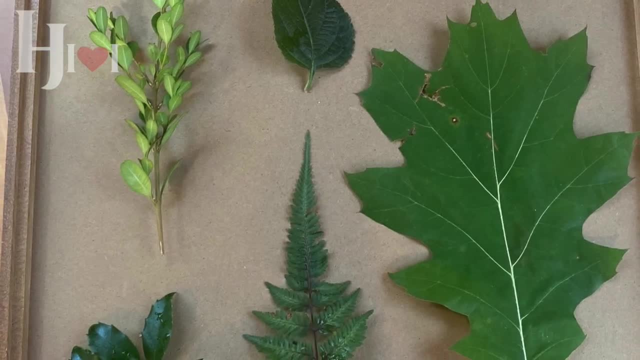 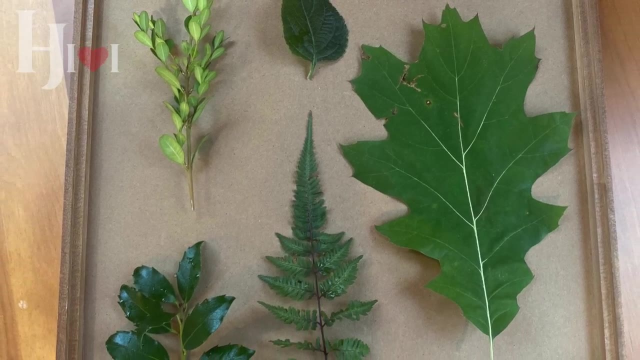 And it can be very seasonal. So you can see, here in the spring you might be noticing all the different kinds of leaves And by putting them on a tray like this and acting like they're very interesting, You know to take the time to point out to the child the differences between the leaves. 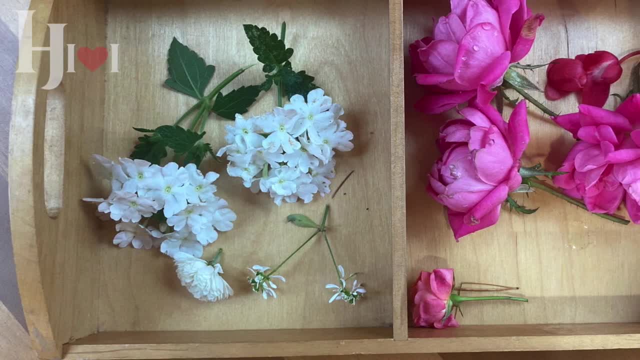 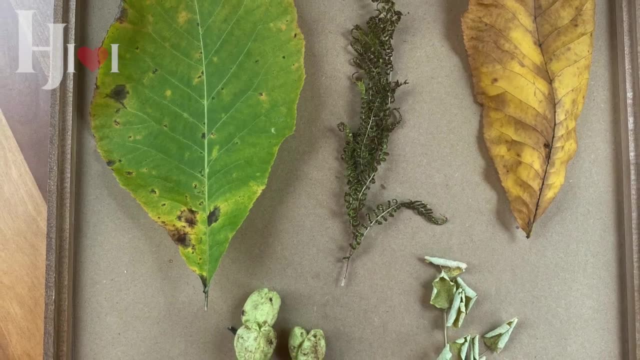 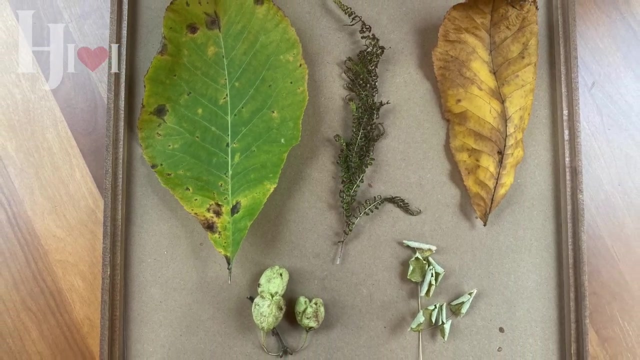 Really can help them understand the benefit of looking closely, Looking for detail. It's a very brain building idea, But it's also a way for them to start to really think about. wow, that outside world is fascinating. It's intricate. The closer you look, the more there is. 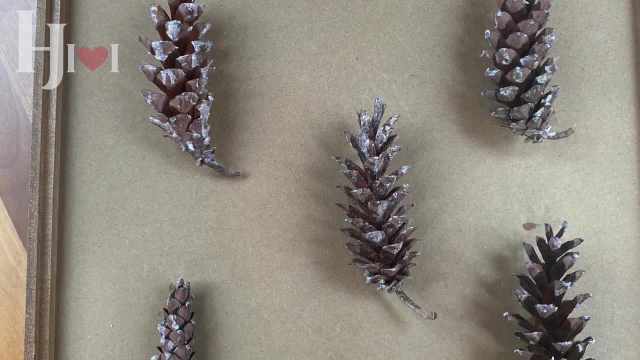 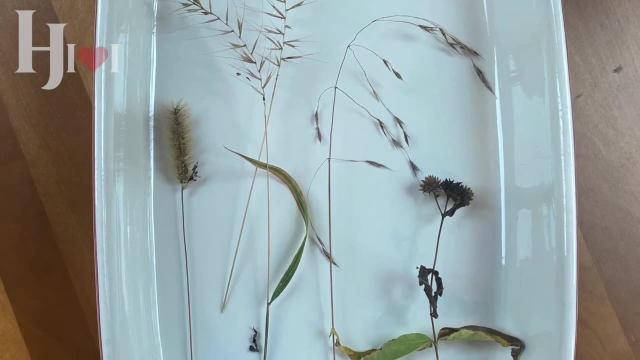 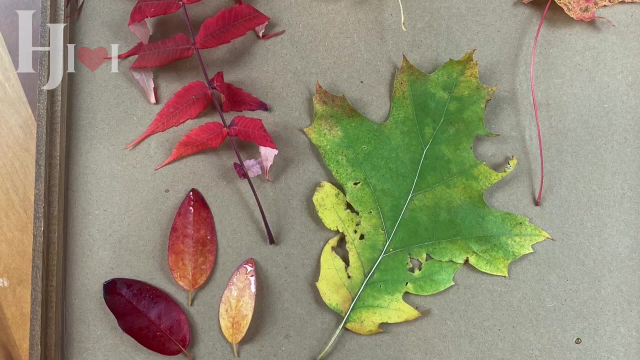 These are big lessons a lot of us are still learning in our life. You can move on from there, So you know you can also, in the fall, You know- point out the beauties of the fall. You can have seed pods, or you're looking at what different things have happened in the fall. 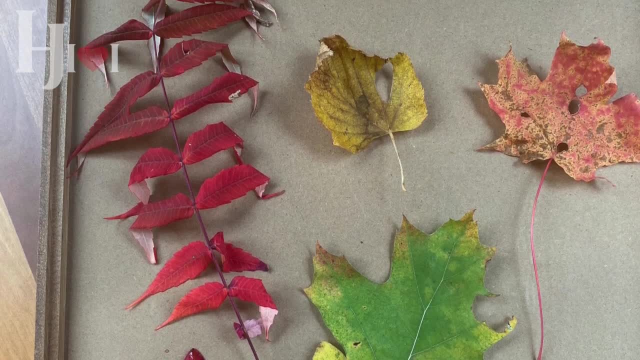 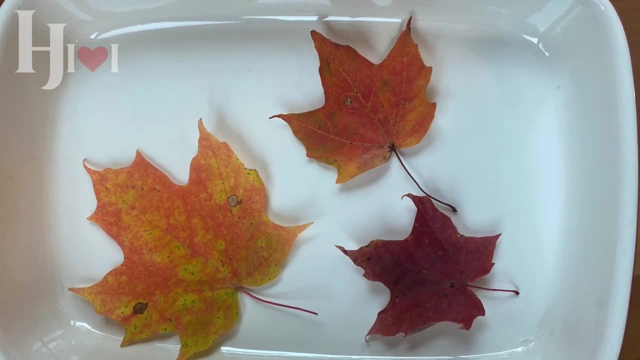 In particular, you can be looking for color changes. It can be just like these are all the different colors that happen. You know. look at these different leaves and how they look. Or you know, in this picture with the white tray. 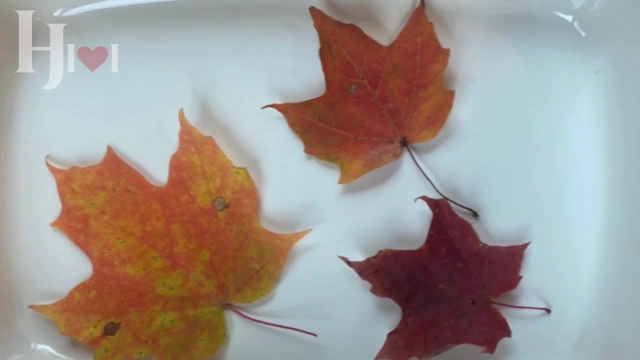 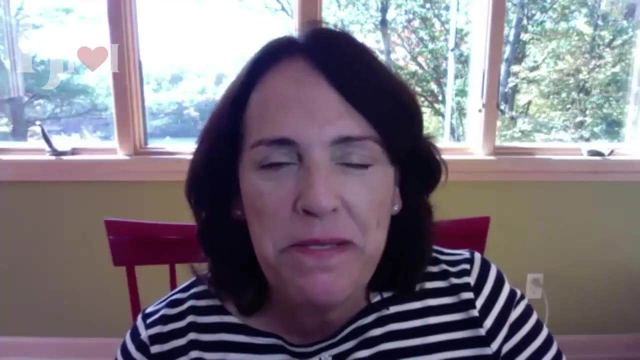 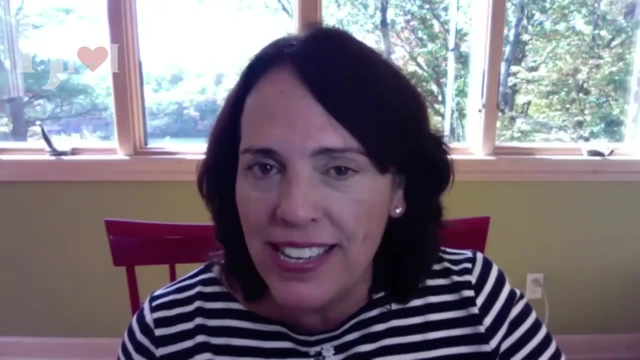 It can be just showing your child how leaves change color, Like the same kind of a tree is slowly changing. Because, again, you know if you watch this, Again, you know if you watched my other video about building brain development in toddlers, you know that I really want toddlers to be able to notice processes. 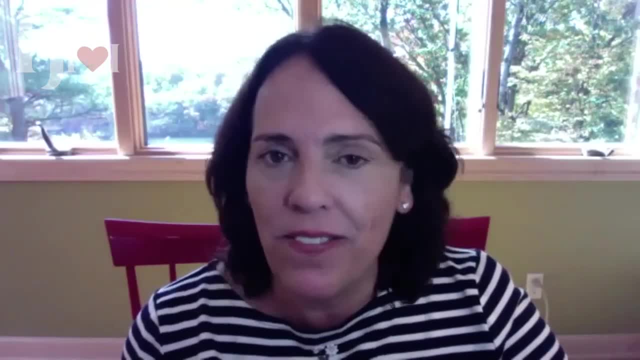 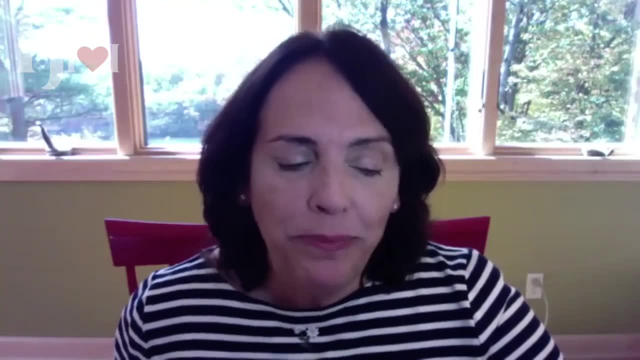 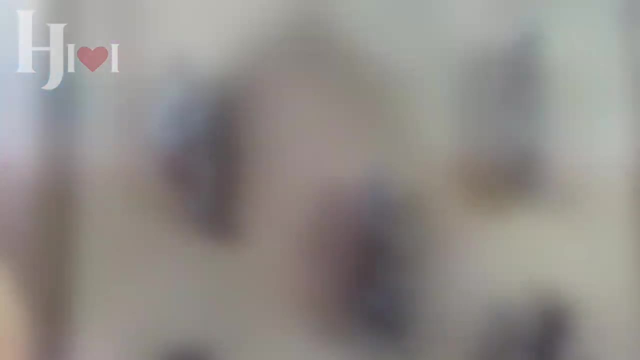 To be able to start to think things through. Not everything is a flash right. Things take time, And what is that process of things changing? So that can be a beautiful way to do this. You can also notice a particular thing. So if you have a young toddler, it could be that one day you're out in the woods and you're like, hey, let's collect pine cones. 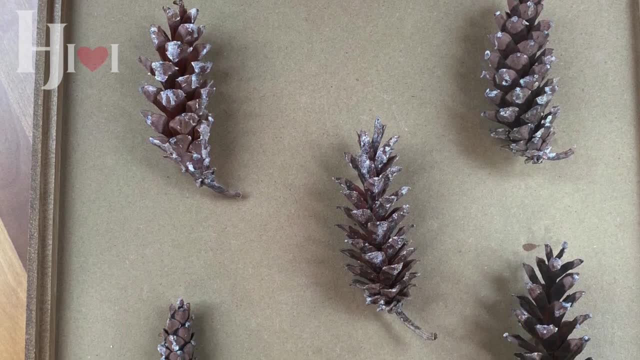 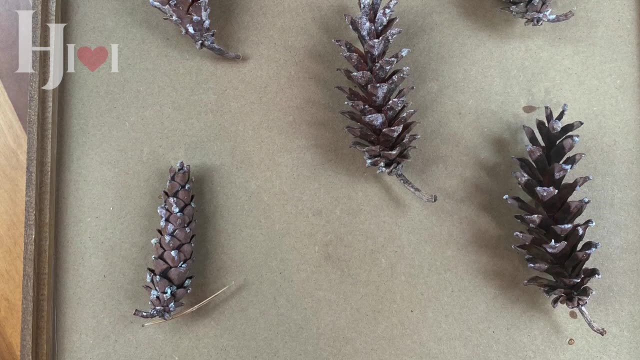 And you bring them home And you're just learning the word pine cone, You're showing them that there's seeds in the pine cone And you're just talking about pine cones. But if you have a little older toddler you might be picking something- like this particular day, where it's kinds of grass seeds. 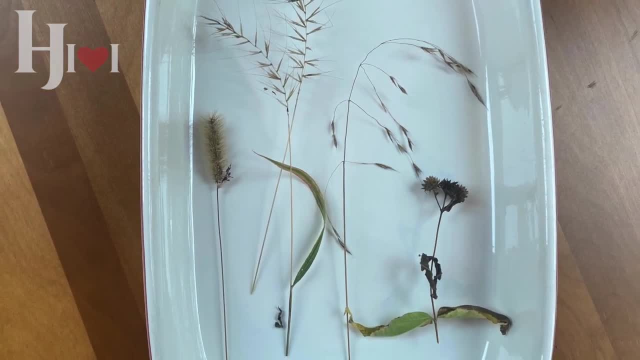 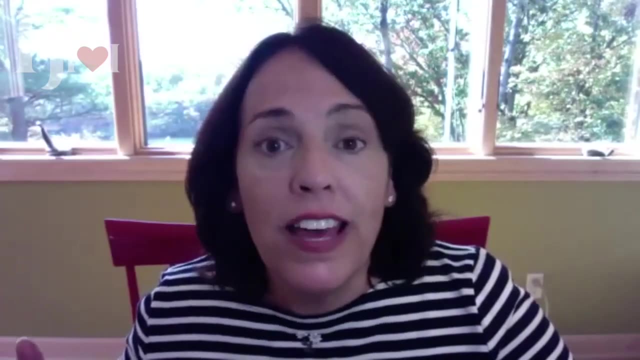 These are different kinds of wild grasses that grow, you know, actually on a property. So bringing them back and just, instead of just them, kind of being a wash of all the things, just saying like hey look, these are all different kinds of wild grasses. 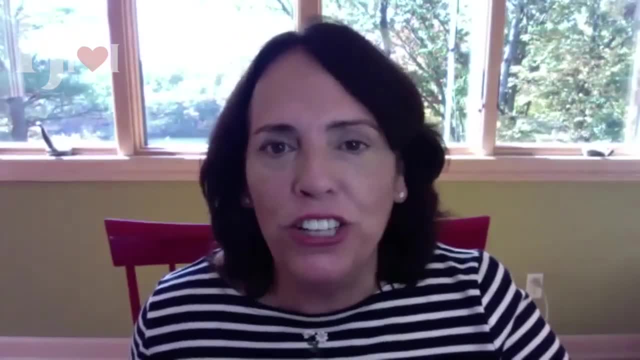 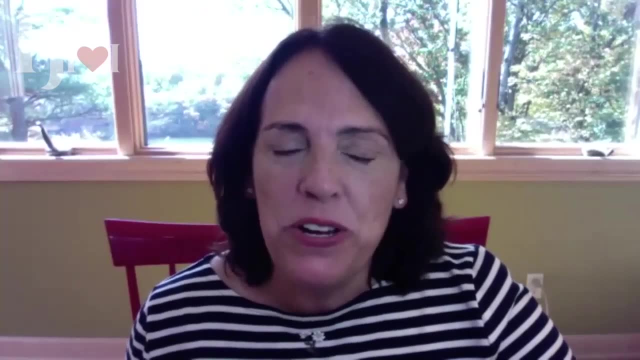 These are all different kinds of wild grasses And look how different they are, Look what variety they are. And this again is you're helping your child to notice detail. You're helping your child to get that feeling for how much depth there is in nature. 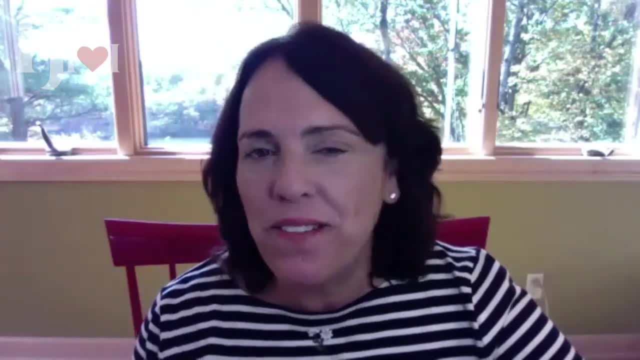 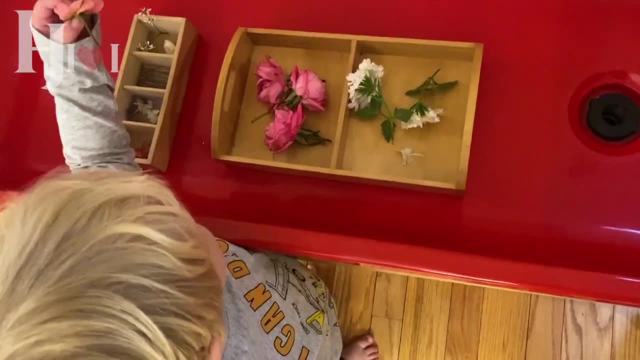 So then you know, obviously you know, if it's spring or you have a great garden, you may be interested in flowers And the thing about flowers or pine cones or whatever is. a lot of kids are going to find these a lot more engaging. 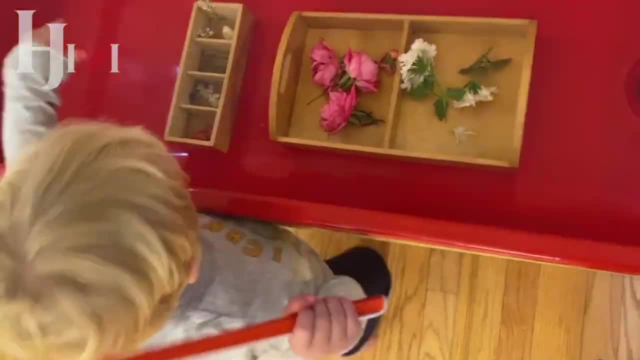 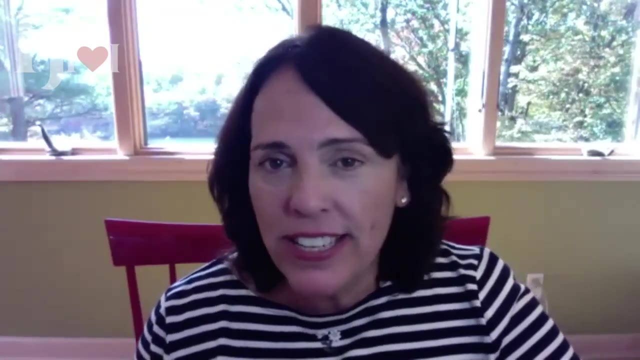 And exciting to work with than just blocks or, you know, whatever you're normally using at your, you know, at your centers to have this variety So you can use it in the idea that you can see in this picture like you're just going to separate. 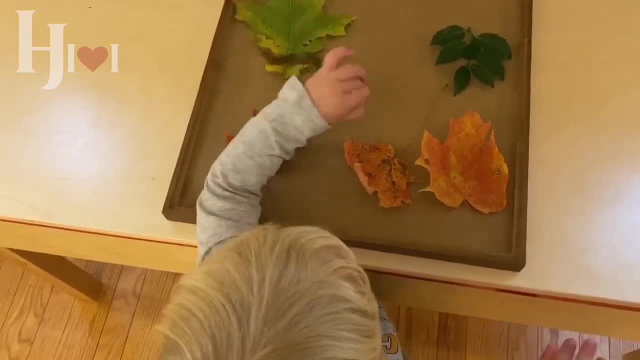 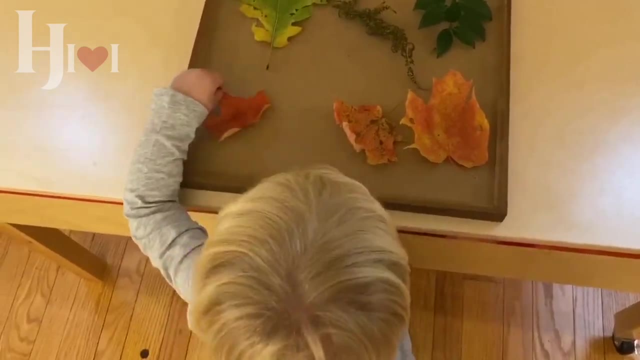 This is a leaf and these are flowers. We're just, we're just making that separation, But it could also be a lot of different things. It could be color right. Like these are pink flowers, These are white flowers. It could be that you're going to do this. 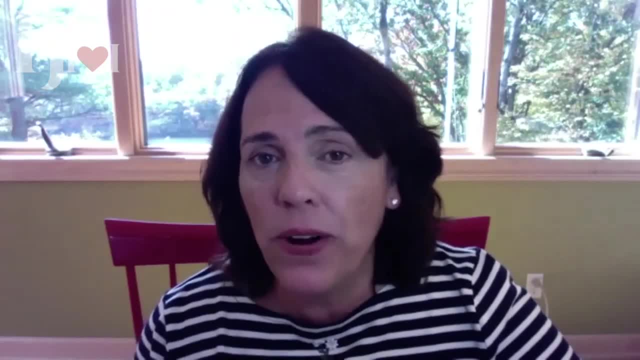 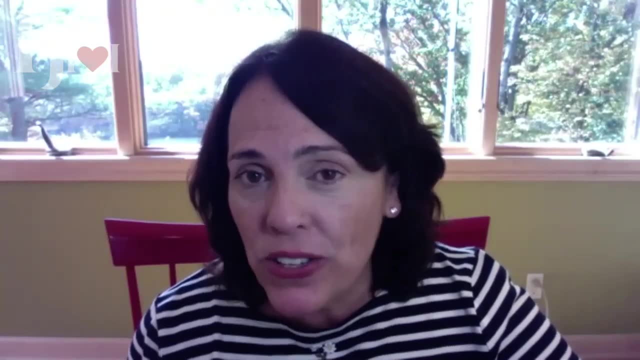 You're going to do something like counting, like where there's one of this kind of flower, There's two of this kind of flower, There's three of this kind of flower. There's all kinds of different ways that you can throw in some sort of skill-based learning. 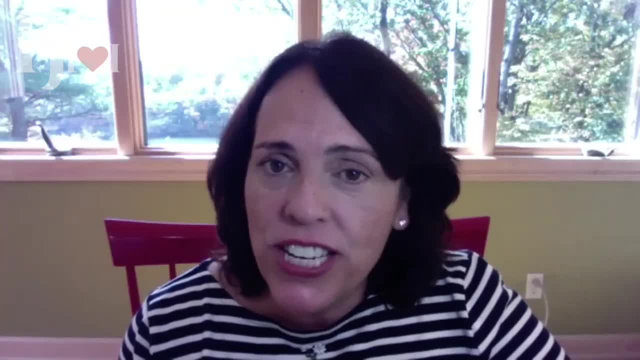 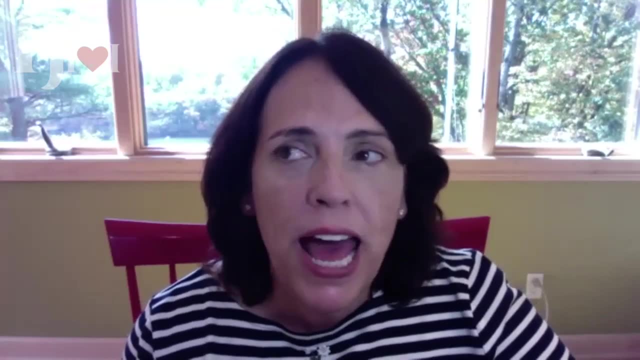 But you're also noticing the beauty of these things. You're taking time to say like: look at this white flower. You know it's really a group of small white flowers. Look at this pink rose. Look how many different petals there are on this rose. 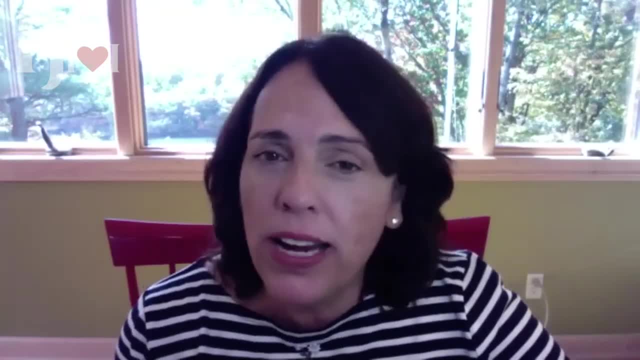 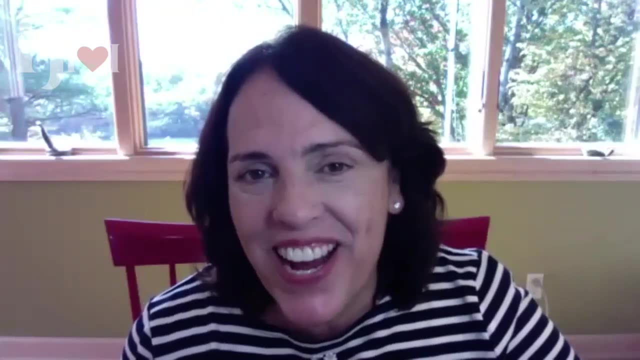 And your kids usually can't. you know, kids are different, So some toddlers might not want to look at this for you know an hour, But just to show it to them for a few minutes of their time when they're noticing it. it's all building up right. 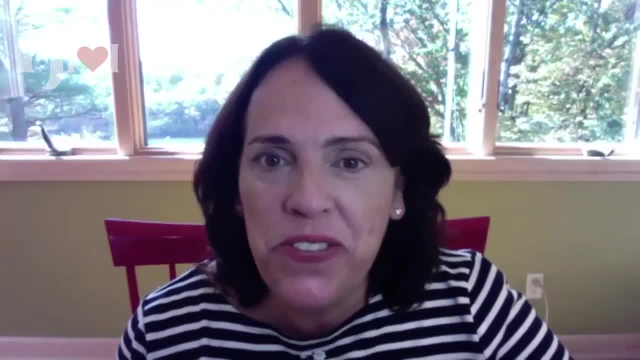 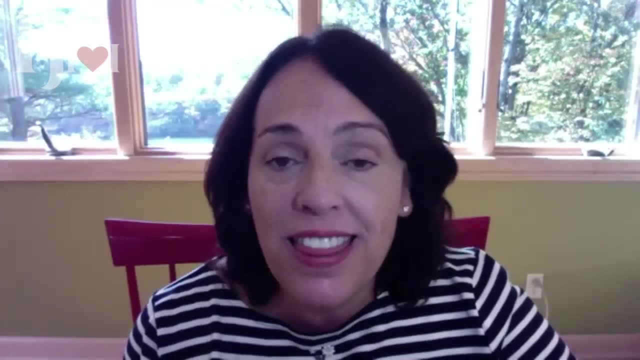 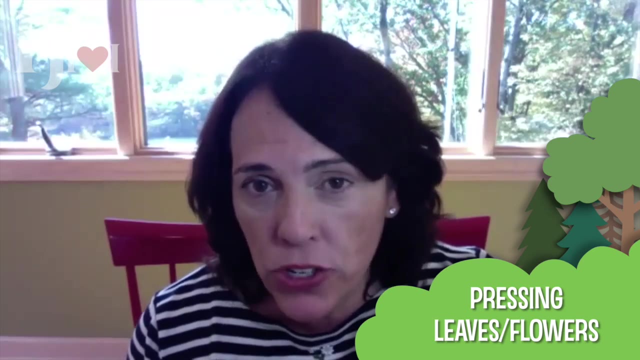 It's all building towards them realizing how beautiful, how complex, how interesting nature is, But helping them to appreciate it themselves, so that the next time they're going by that they're noticing these things too. So a thing that a lot of toddlers are going to really enjoy. 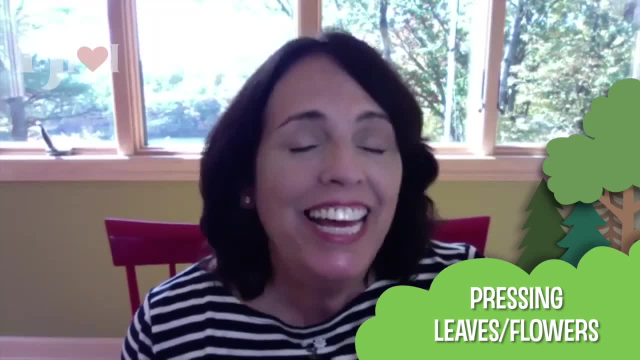 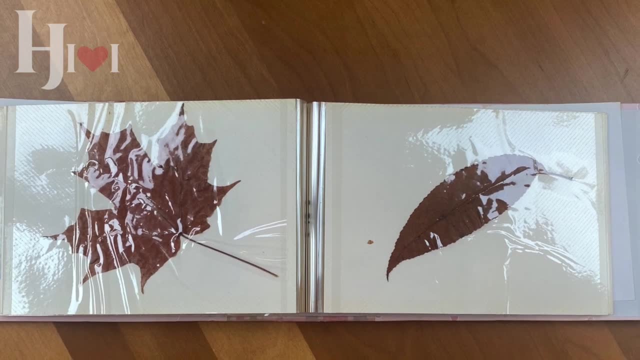 is the idea of pressing leaves And, you know, this is something they really can do themselves. It's something that they really can do. But if you look at this book, this is actually a book my daughter did you know 29 years ago, or 28 years? 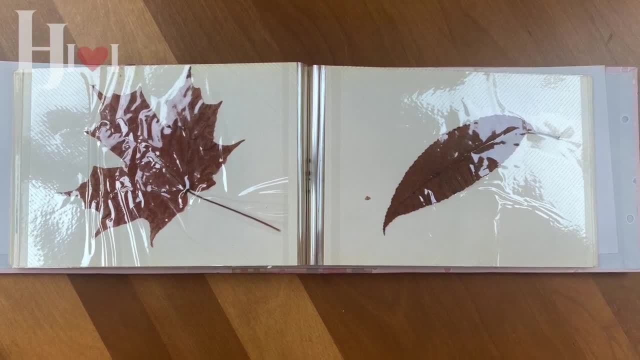 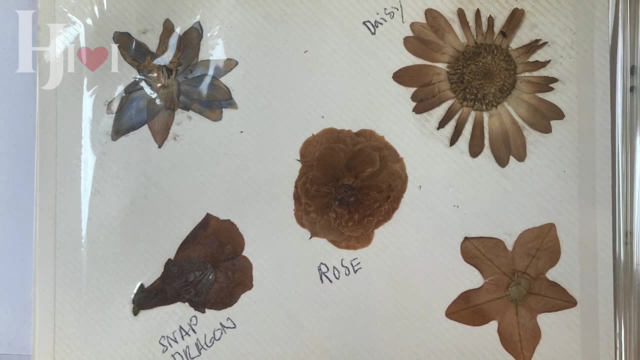 And you can see as a toddler, what she's actually doing is just putting you know, leaf a leaf on the sticky page And you know, that's it. But as she's older- I think this next picture is when she was six- she can put a variety of flowers on there. 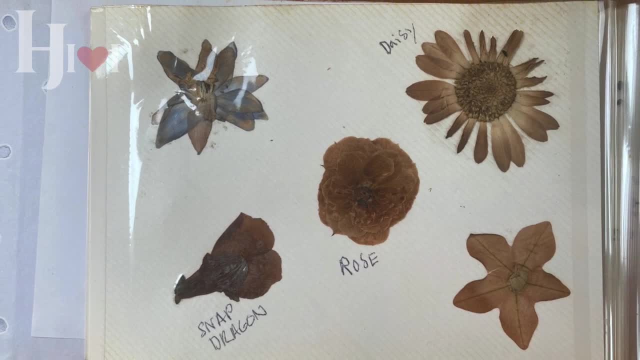 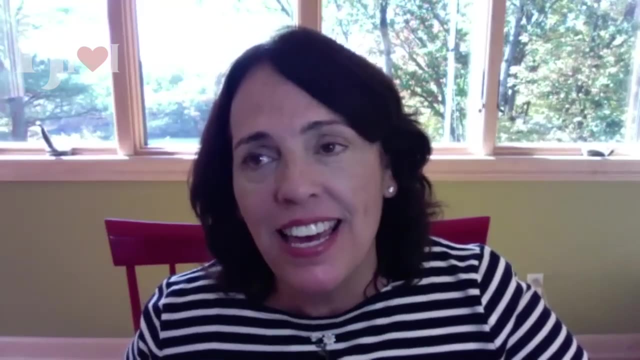 She can even write. you know their basic names. This is something that you know. you just put a few in a year And it's a very precious thing then, when your child is much older, to look back and see that every year. you know. 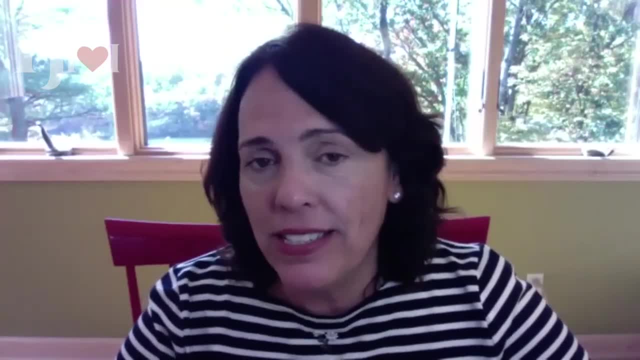 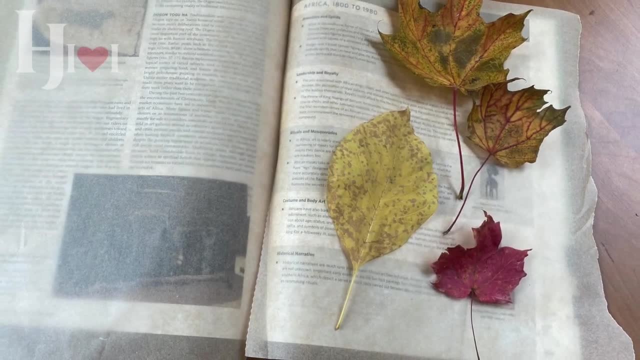 or every other year. whatever you do that, they did press some of these leaves. You can see here that I'm just going to briefly show you with these pictures how to do it. So you could use parchment paper, You can use wax paper. 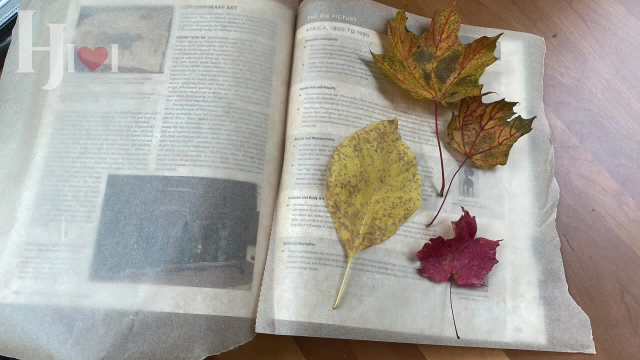 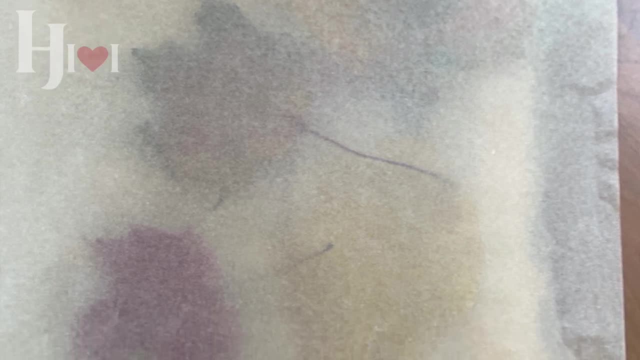 You can actually use no paper, but it sometimes ends up with a little mold, And the reason you want to do this is you want to get as much water out as you can before you put it in your booklet, so you have the least likely chance of having it mold. 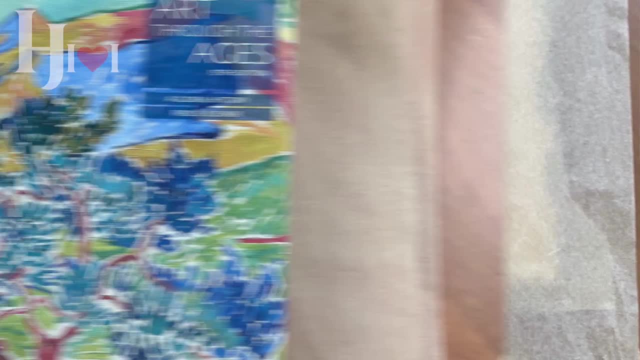 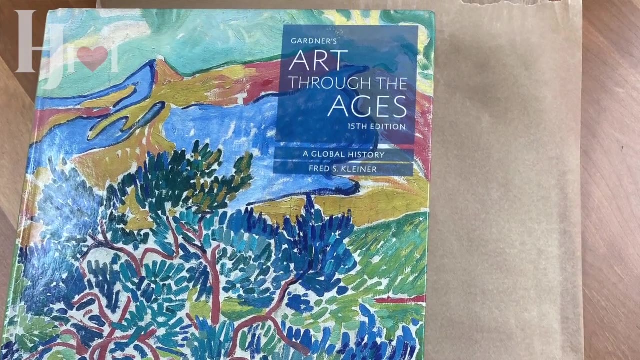 So by putting parchment paper on either side of the book, then the child. all they have to do is close the book. If you use a thick enough book, just the weight of that book and if you did your pressing down low will actually be enough. 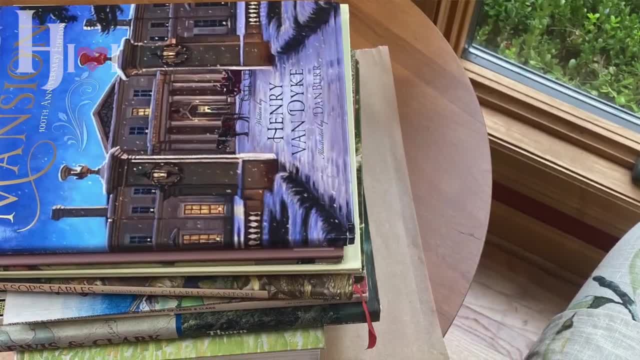 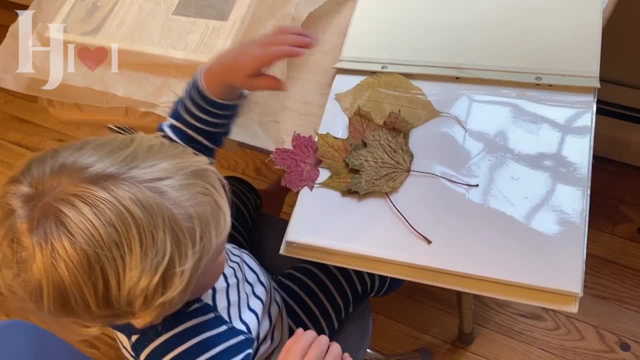 But you can also try just putting more books on top of it, right When it's ready. you know a toddler, even a young one-year-old. you can take that leaf out and put it on the sticky page of a binder. 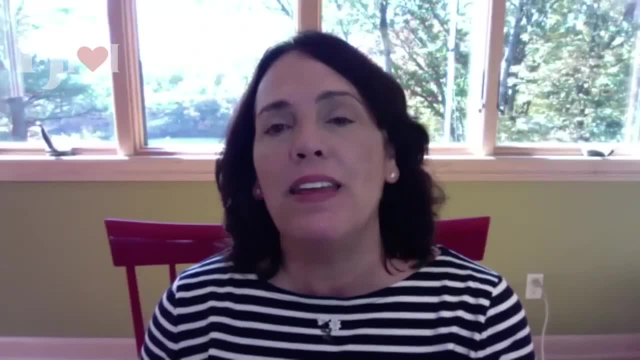 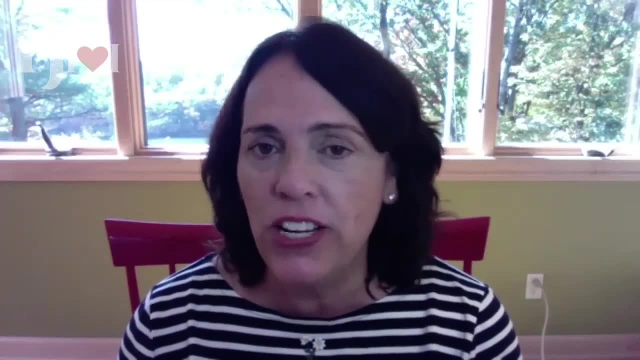 You can see here in this little video he's doing it too- and then press it back. There's so much you can do with that. You can just save it. I've also used it to go through later in the winter and do things like just get kids to basically understand. 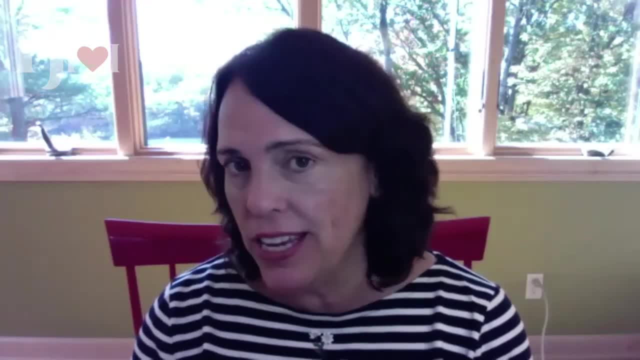 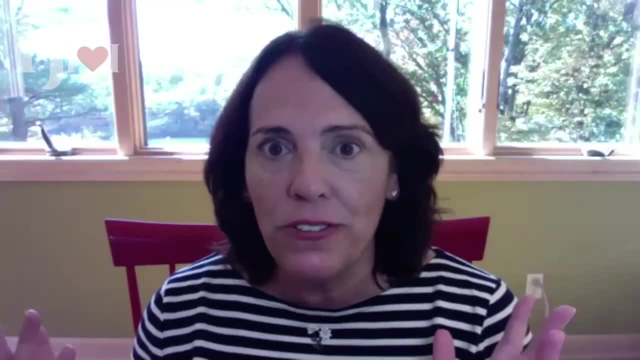 oh, that's a maple leaf, that's an elm leaf, that's an oak leaf. You can also use it to count The colors. don't last forever, but early on you can you know, the first year or something you're still going to be able to use it for a color. 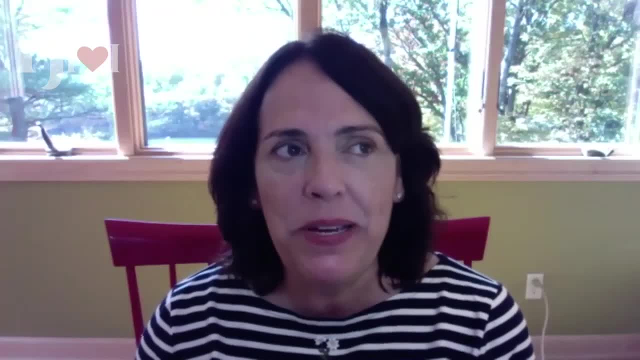 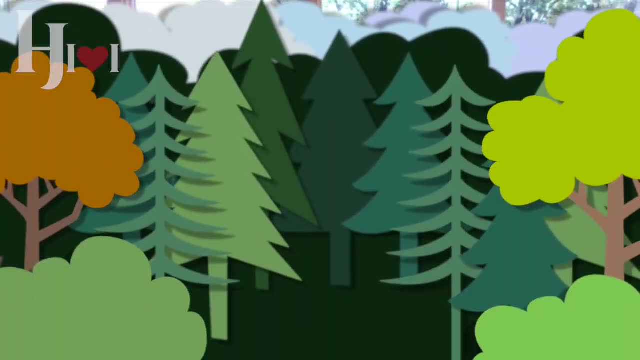 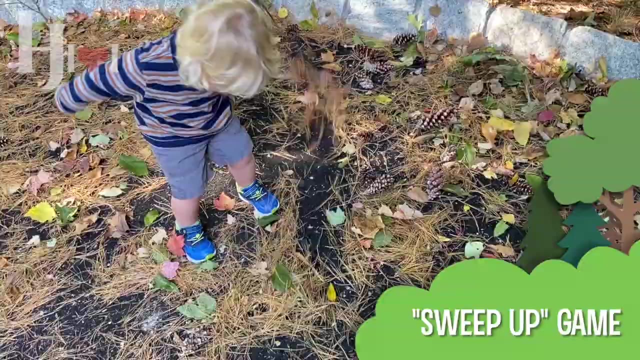 And because they actually made it themselves, they tend to find it to be just really great, something that they enjoy doing. So, anyway, maybe you'll like that too. All right, so the last activity I have for you today is this idea of letting your child take an evergreen branch. 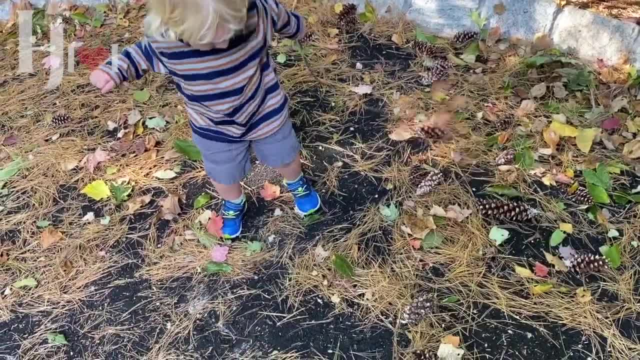 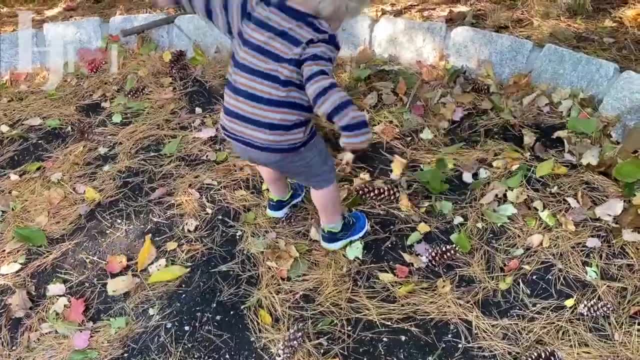 and use it to sweep with. Something about this is just so intriguing to toddlers. I'm not even sure I can understand The passion that a number of my toddlers have had for this activity, But whether you do it in the driveway, on a nature trail or in your backyard, 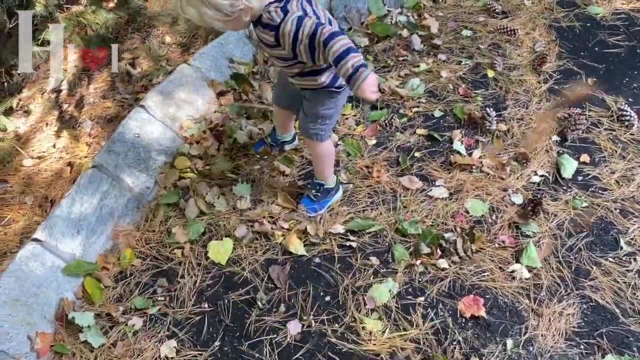 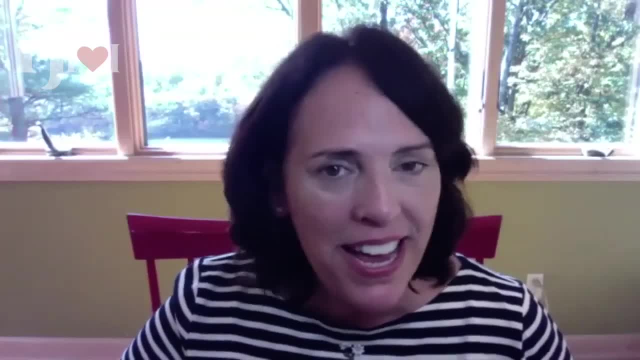 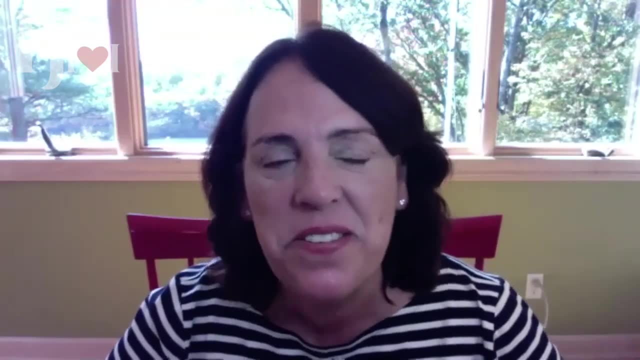 just using that evergreen branch to sweep up pine needles or other things. I think it's the sound. you know the sound that makes and you know just the vibration maybe, But it's something that you definitely want to give your child a chance to see if they also are going to enjoy that. 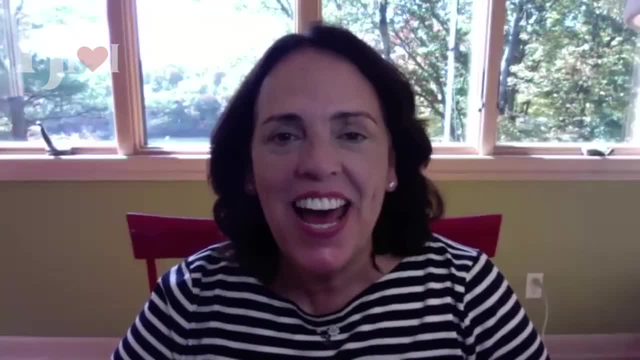 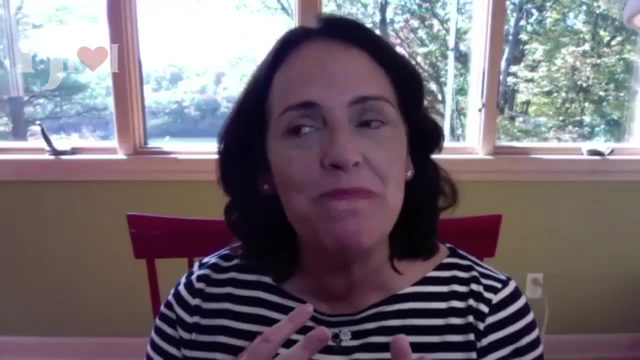 in the way that I've seen so many of my toddlers. Thank you so much for listening. Obviously, this is something I feel very passionate about: This idea of getting this bond between you and your child, but also between your family and nature.